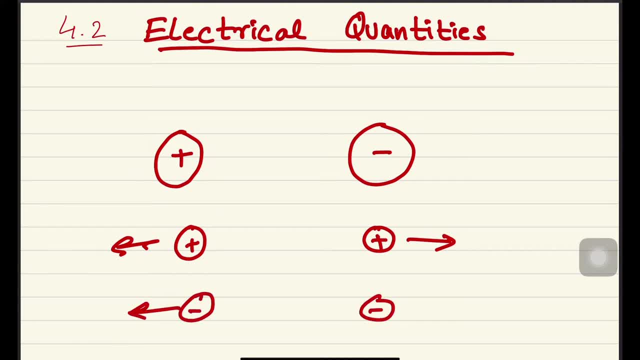 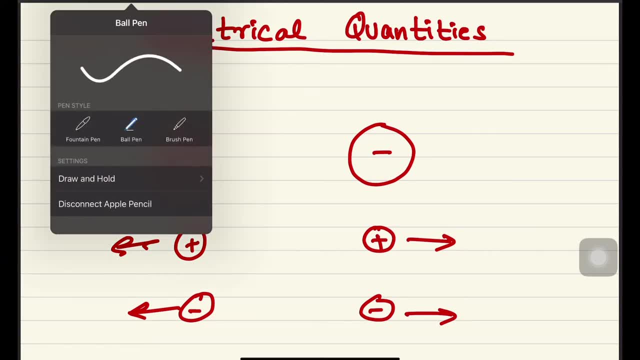 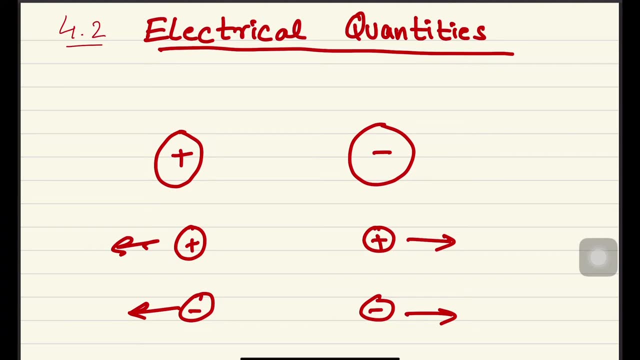 and if we have two negative charges in front of each other, they'll also rebel. it's basics, just the basic phenomenon. so we can say that the like charges, they repel each other and the unlike charges attract each other. so from the introduction of charges we'll 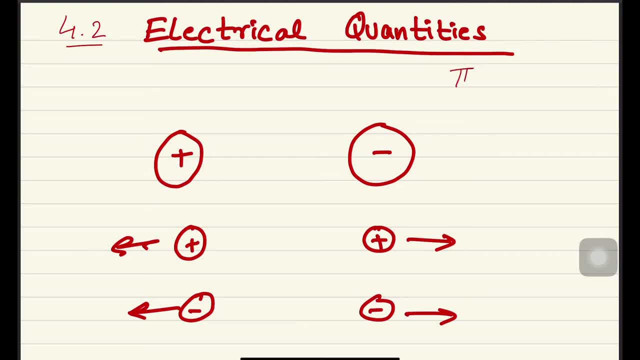 have to. just we have to. we have to say that the like charges. like charges means positive, positive or negative, negative. so the like charges repel each other and the unlike charges attract each other. unlike charges attract each other. for example, positive and negative charges, they will attract each other. 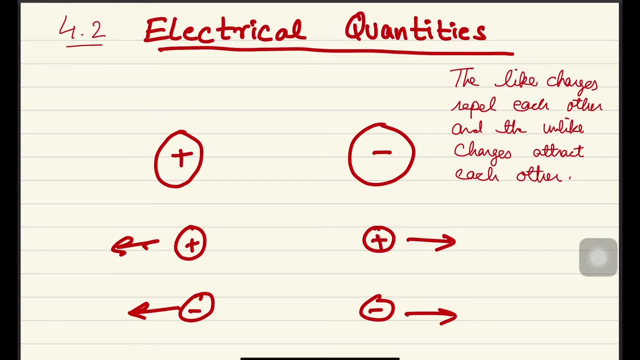 positive positive charges and negative negative charges. they will repel each other. so that's the basic phenomena of the charges. now we have to discuss about the force by which these charges are attracted towards each other or developed by each other. the name of that force is electrostatic. 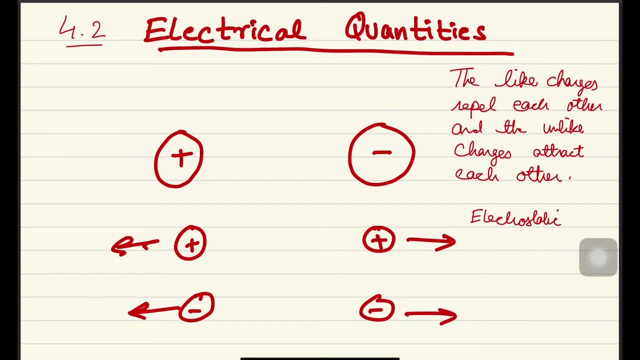 force, electrostatic force. so if the charges are being attracted towards each other, so we will call that the electric electrostatic force of attraction. if the charges are being repelled from each other, we will call that force, as the electors, electrostatic force of repulsion. all right, now we will discuss. 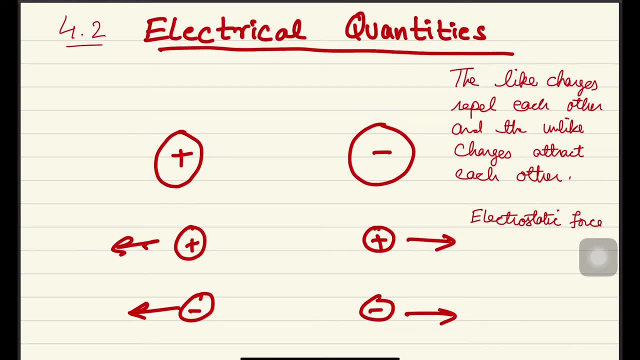 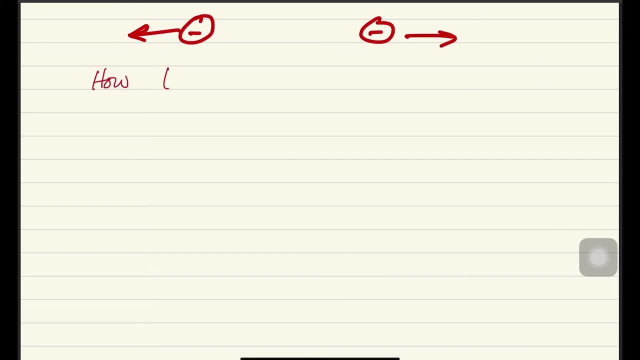 how the charges are moved from one object to another object. okay, how the charge, the charge flows. so the charges, they flow from one object to another by one phenomena and that phenomena is friction. so the charge flows from one object to another with friction. for example, if we have 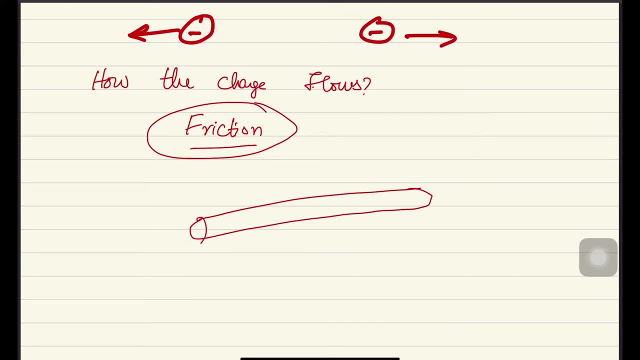 an insulated rod and we rub this insulated road on a a piece of cloth. let's suppose this is the piece of cloth. so what will happen? let's suppose on this road there are 100 positive charges and 100 negative charges, which means that initially this rod is neutral. neutral means an object will be neutral if it has equal number of positive and 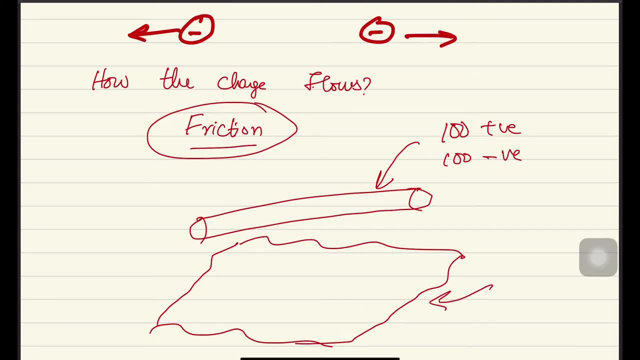 negative charges. okay. and also, let's suppose this cloth: it also has 100 positive charges and 100 negative charges. okay, we can say that initially these two objects are neutral: the piece of cloth and the iron iron rod or any any glass rod, basically not the iron road class, or we are talking about. 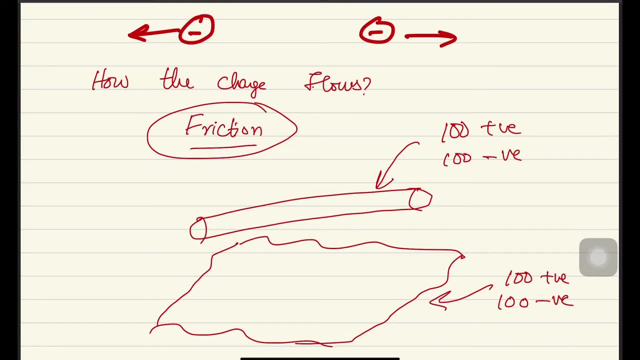 the insulators here. i'll explain you in detail later. so they have 100 positive charges and 100 negative charges. this cloth piece also has 100 positive charges and 100 negative charges. so when we rub this glass rod on this piece of cloth, what will happen? some charges will be transferred from this. 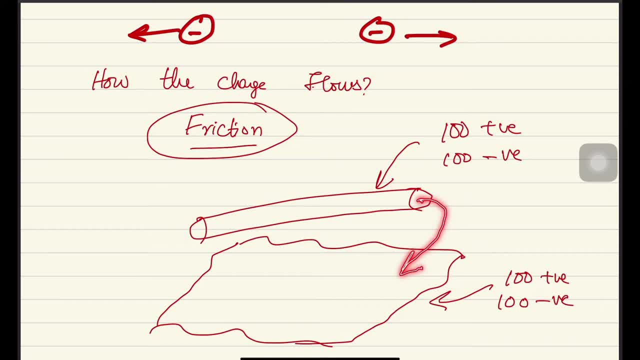 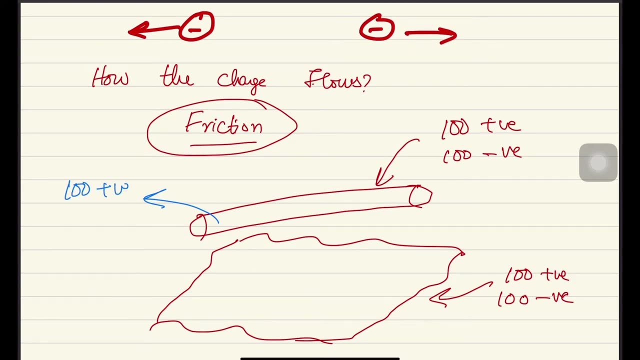 glass rod to the cloth. when i say charges it means some electrons will be transferred. so after rubbing the electrons will become, for example, this glass rod, after rubbing, will have 100 positive charges and let's suppose 90 negative charges. so you see it has the deficiency of negative. 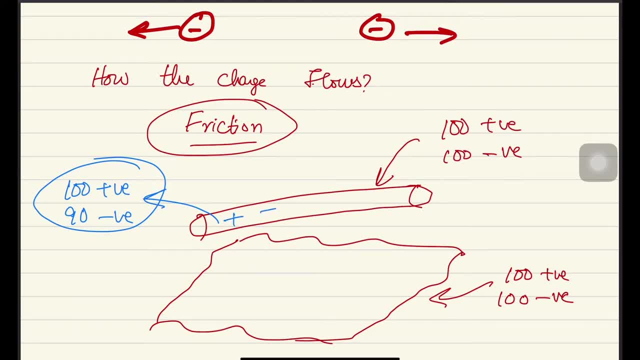 charges, which means, as a result of that, this rod will become positively charged. okay, similarly, on this cloth there were 100 positive charges and 100 negative charges. now, since 10 negative, 10 negative charges have been transferred from the rod to the cloth. so this cloth has. 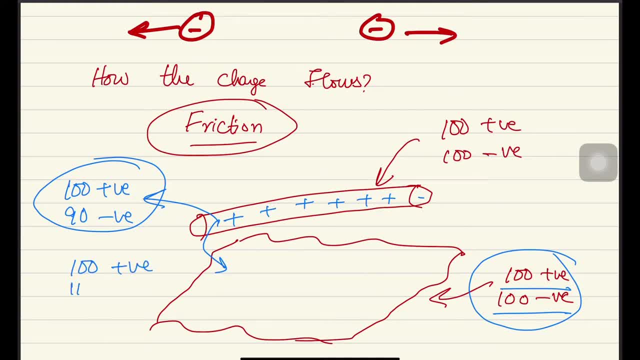 100 positive charges but 110 negative charges, due to which it will have negative charge on it. so that's the phenomena of friction, by which the charges move from one object to another. okay, and this happens due to the friction. okay, now we have to discuss about 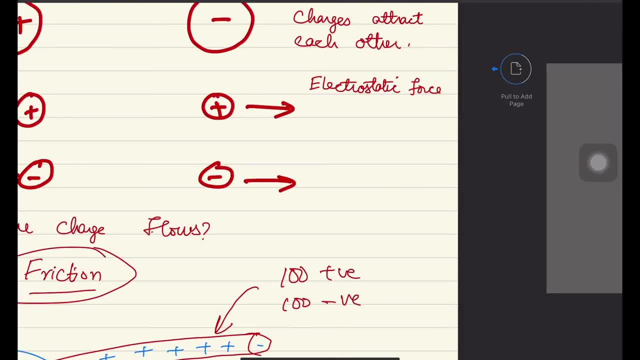 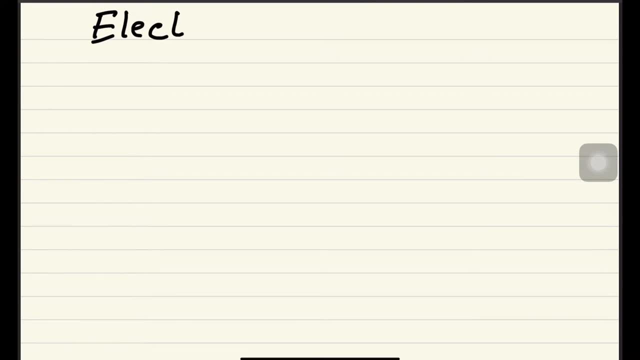 electric field. electric field is an electric field rupturing section of air торточ이 electric field, so electric field. if I define the electric field, I can say that it is a region or space. it is a region or space where a charge experiences some electric force, some electric force. it could be electric force, it could be electrostatic force. 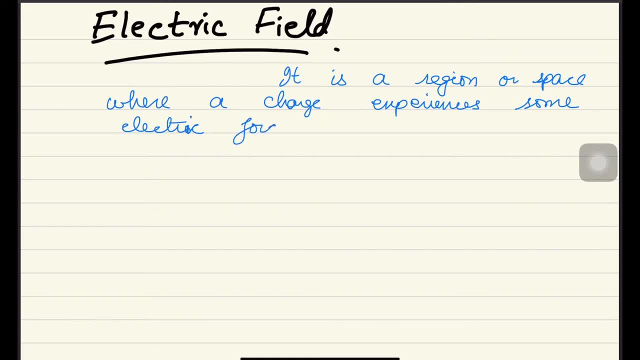 of attraction or the electrostatic force of repulsion, so that region is called the field. for example, I have a positive charge and the range of this positive charge is till here. okay, so if I place some negative charge over here at this point, then they, these two charges, will attract each other. 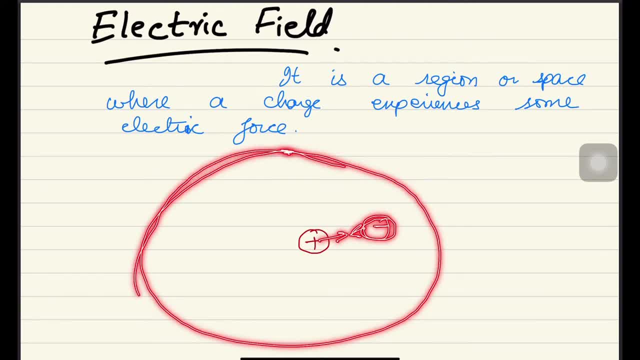 okay, so this region where this positive charge has its influence, this region is called the electric field. all right, so if I place a positive charge over here, let's suppose the range of the influence of this positive charge is within this circle. so this circle, the region, this 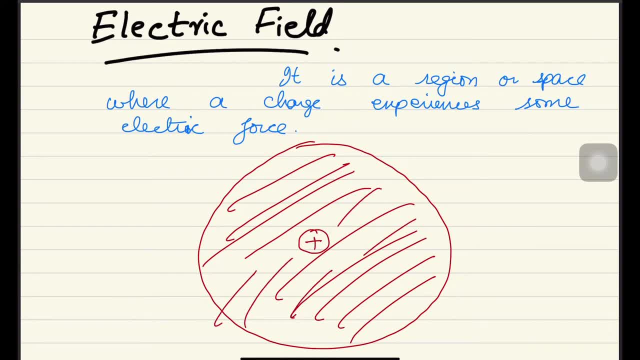 region is called the electric field, where I will put any charge and that charge will experience will experience the electric electrostatic force of attraction or repulsion depending upon the nature of the charge. for example, if I put a positive charge over here, it will be repelled, and if I put a negative charge, 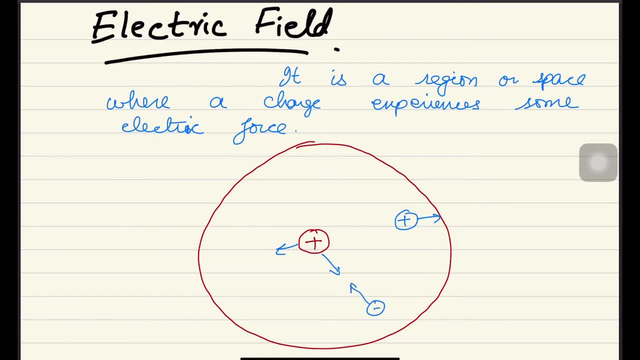 over here, it will be attracted towards this positive charge. so that's the simple phenomena. okay, so that's the concept of the electric field. um, yeah, that's it now we have to discuss. okay, this is the electric field due to a point charge. this is the. this is considered to be a point charge. so that's the example of 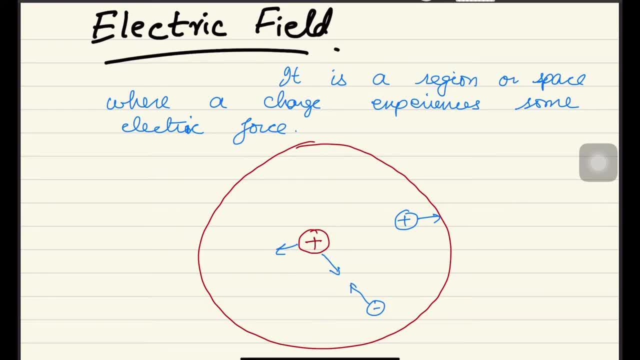 the electrostatic electric field due to a point charge. I'll just mock it up so you will remember that because it's in your specification. so: Electric field due to a point charge, you a point charge, okay. so that's the example of electric field due to a point charge. now we 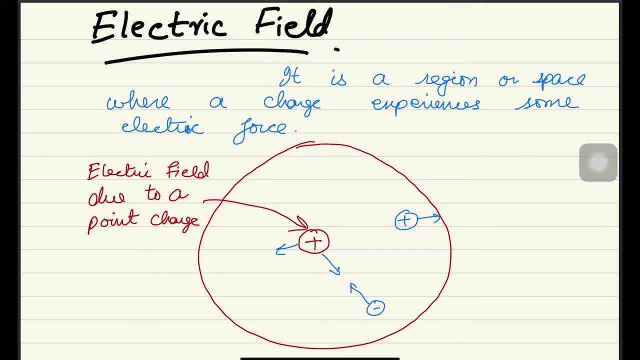 have to discuss the example of an electric field due to a charged conducting sphere. okay, there's a difference between them. this positive charge is just considered to be a point charge. it means it has a negligible radius. in fact, it has no radius, it it's just a point charge. now we have to discuss. 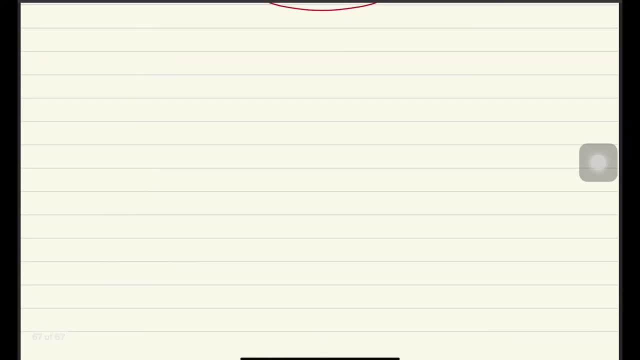 the charge around the sphere. so I'll draw a sphere first of all. let's suppose this is the sphere, let me just draw it. let's suppose this is sphere, okay, and it has a positive charge on it. on the surface of the sphere there's a positive charge. there you go. now you have to remember that. 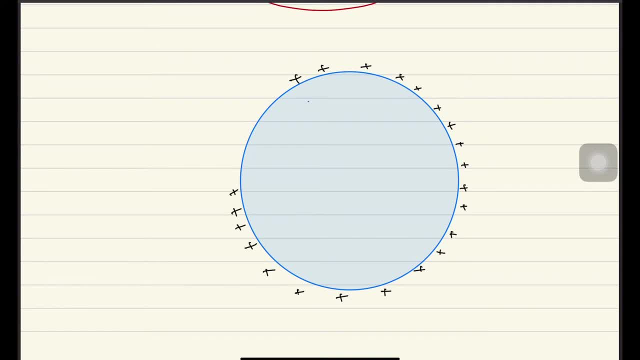 we are talking about the positively charged or any charged sphere. so in this case we have the positive charge is spreaded on the sphere, but you know what? there is nothing inside the sphere. there is nothing inside the sphere. so if you put a point charge, let's suppose you have a point charge and 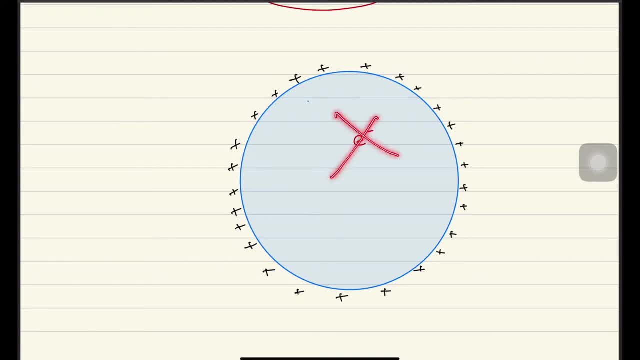 if you put an electron over here, nothing will happen to this electron. there is no force of attraction or repulsion. so that's the difference between a point charge and the charge in a sphere. although if you put an electron over here at this position, then you will see a, an electrostatic force. 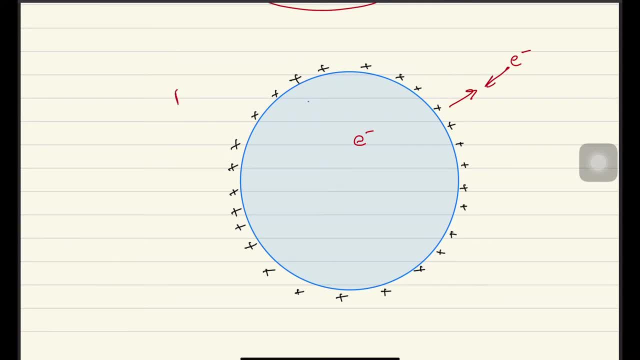 of attraction, and if you put a positive charge near to this sphere, you will experience the electrostatic force of repulsion. all right, so that's how the we can explain the electric field around the positively charged sphere. the only difference between the point charge and the and the sphere is that in the point charge, 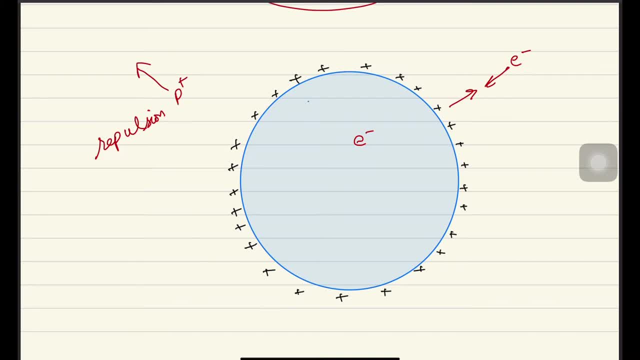 the radius is zero and in a charge conducting sphere there is some radius, but within the sphere there is no charge. there is no electric field. in fact we can. if we place a charge over here, it will not be affected by any electric field. so the electric field strength. 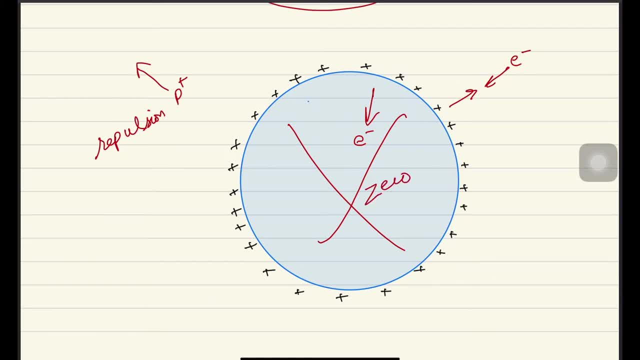 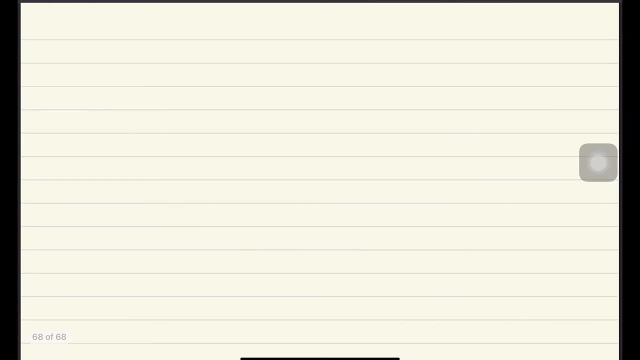 over here is zero, which means there is no electric field between them. now the next example that we have to discuss about the electric field is about the electric field in the charged parallel conducting plates. okay, so I'll just write it over here: electric field between charged conducting. 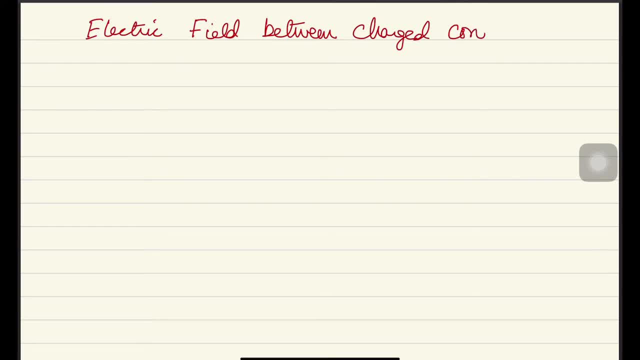 plates. so if you place two plates, for example, that's one plate, here's another plate. now there's a positive charge on this plate and there is negative charge on this plate. now the question is how that positive and negative charge will come onto this plate. it means, like we can explain it like: 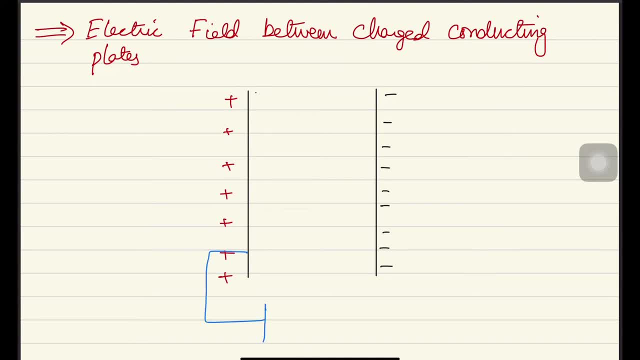 this: that this positive plate is connected to a battery- the positive terminal of the battery- and this negative plate is connected with the negative terminal of the battery. that's the positive terminal, that's the negative term in any, in every battery, there are two terminals: positive terminal and the negative terminal. so this positive plate, since it is connected with the positive terminal. 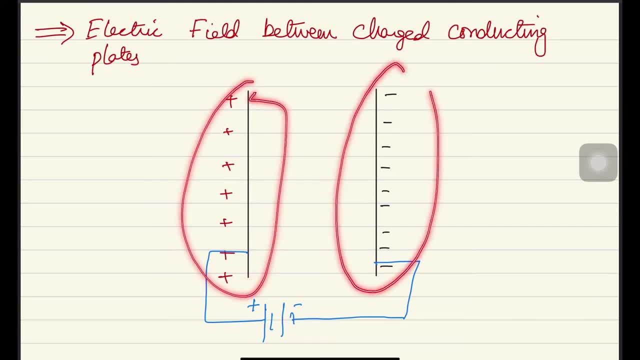 of the battery, so it has positive charge on it. and this plate, since it has been connected with negative charge, so it has positive charge on it. and this plate, since it has been connected with negative charge, so it has positive charge on it. and this plate, since it has been connected with. 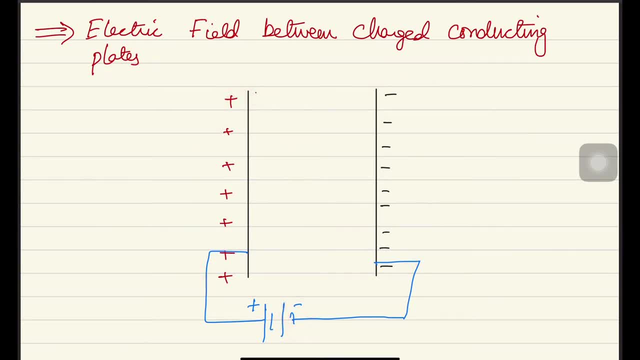 negative terminal of the battery, so it has negative charge on it. okay, so that's how these plates will become positive and negative charges charged. now we have to check the direction of the electric field between these two conducting charged plates. so in order to show that we have 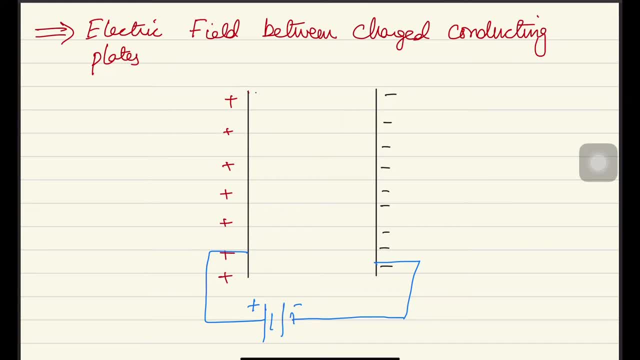 to draw some arrows. so on the edges of these conducting charge plates, we will see the direction of the electric field from the positive plate towards the negative plate. okay, and within these, uh, within these conducting plates, now, within these conducting plates, it will be straight like that. so that's the direction of the electric field between these two conducting plates. there you go. 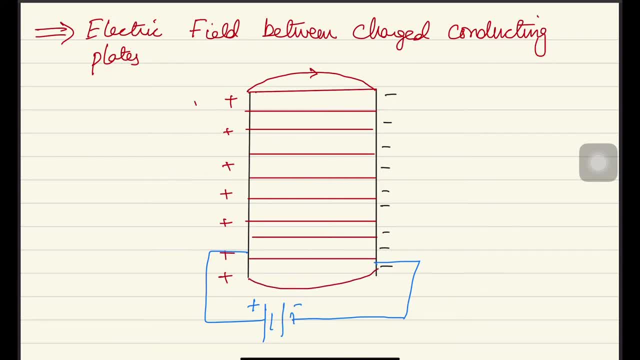 okay, now i'll just draw them the errors, in order to represent the direction of the electric field. so, when there are two charge conducting plates, the direction of the electric field is from the positive terminal of the battery towards the negative terminal of the battery. all right, so these are the this. these are the three examples of the electric field due to, first of all, we have 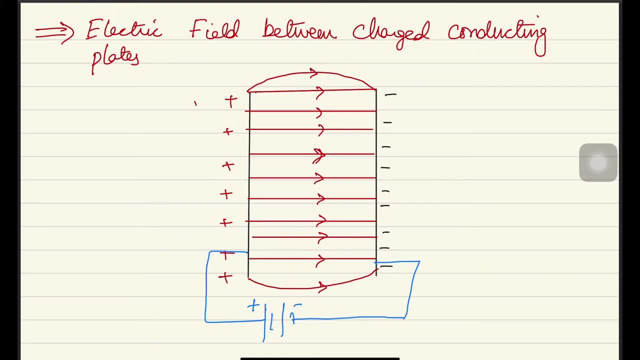 discussed about the uh, about the electric field due to point charge, then the charge conducting sphere and thirdly- we have explained it- between the two conducting positive, between the two conducting charged plates. one is positive and the other one is negative. now, one thing that you have to note down over here is the strength of the electric field in this whole region will be. 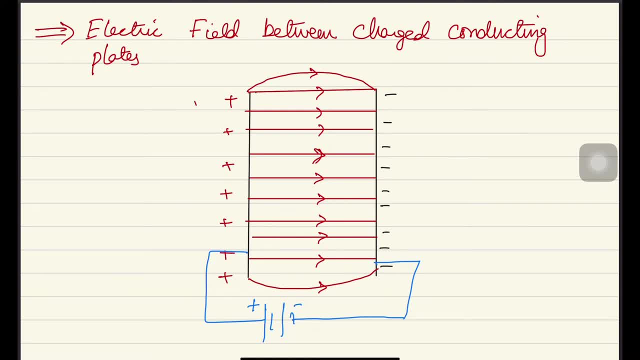 constant. for example, strength means the electric force. for example, if i place an electron over here, here, here, here, here, at like random places, So the force, the electric force that will be exerted on these electrons will be same in all places, okay, 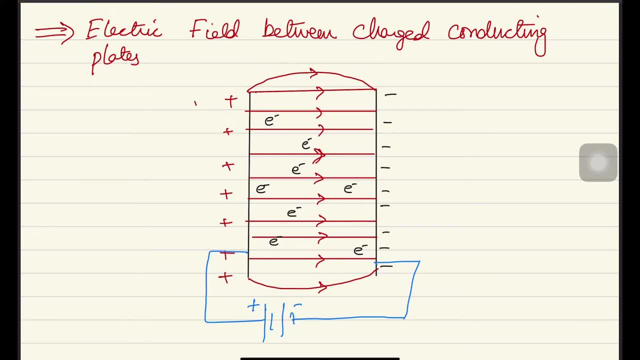 The force acting on these electrons will be same at all. The strength of the electric force will be same, why? Because these electric field lines are at equal distances from each other. These are the parallel straight lines. They are at equal distances from each other. 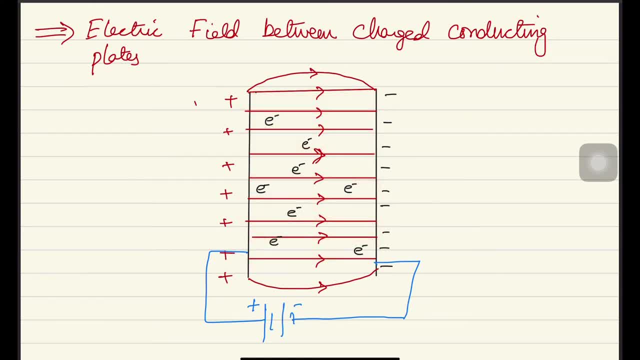 since they are at uniform distances from each other. it means the electric force is constant. The force that is being acting on the charge is constant. Okay, That's very important point that you have to keep in mind. Now we have to discuss about the conductors. 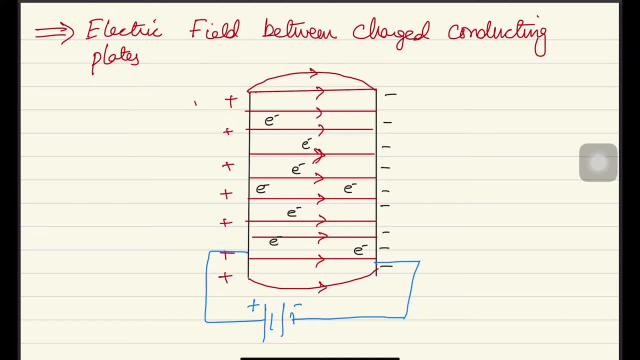 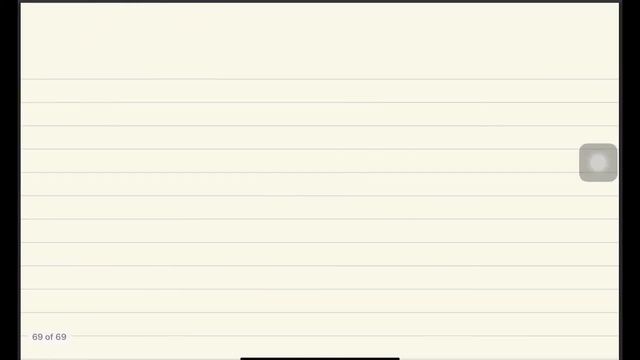 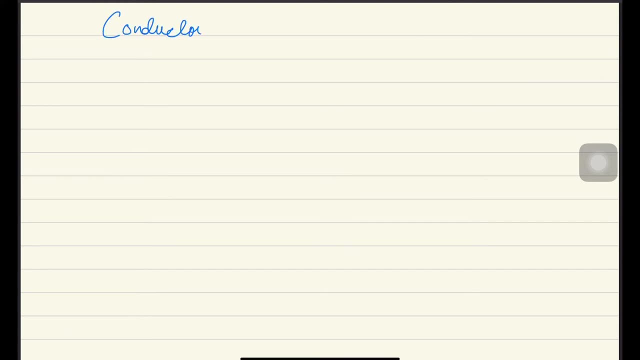 and the insulators, and then we will differentiate between. we'll discuss an experiment by which we'll differentiate between the conductors and the insulators. Okay so, conductors and the insulators, Conductors and insulators. So it's quite simple. 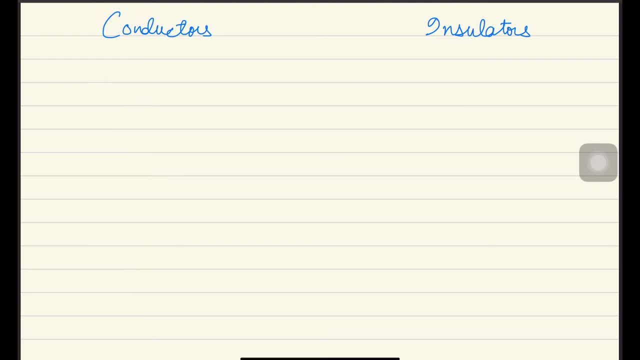 Conductors are the objects through which electricity, through which the current can pass, or the charges can flow, But the insulators are the objects through which the current cannot pass. That's the only difference between the conductors and the insulators. So the objects. 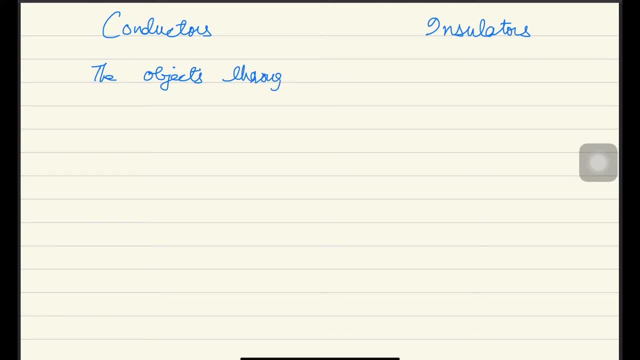 through which current passes are the conductors, And insulators are the ones, the objects through which the current is, Through which current does not pass. Current does not pass. are the insulators, Or the insulators, If you know, multiple Earths. 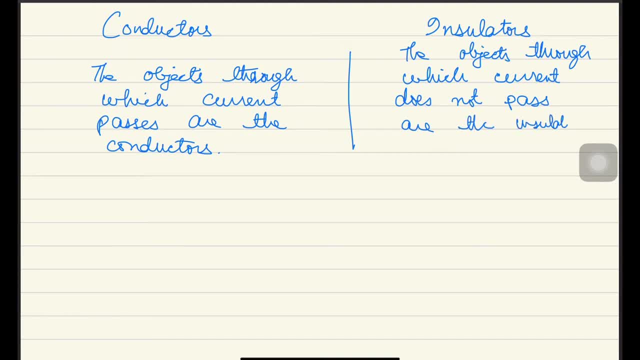 So this will also apply to the heat. So the object through which the heat passes- They're normally the conductors- And the object through which the heat passes- in a commonhalse, Guys burning all good which the heat does not pass, that the insulator. but since we are talking about the electricity, 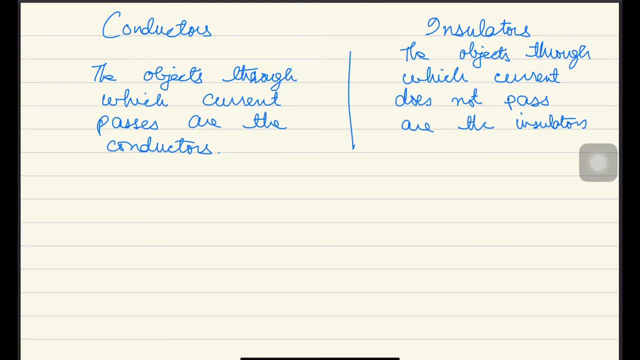 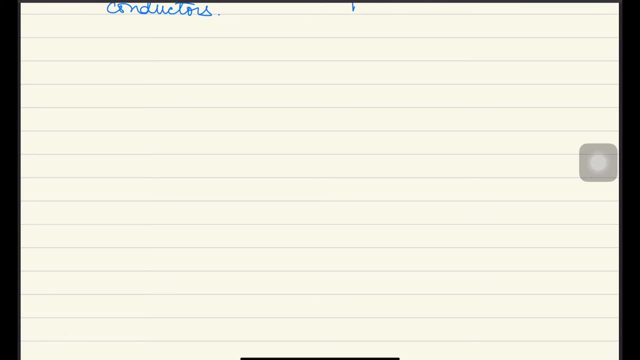 in this topic over here, so i'll only um consider electricity. okay, now let's design an experiment through which we will identify which object is a conductor and which object is not a conductor. so for that purpose i'll just draw a simple circuit and for example, this is a: there's a light. 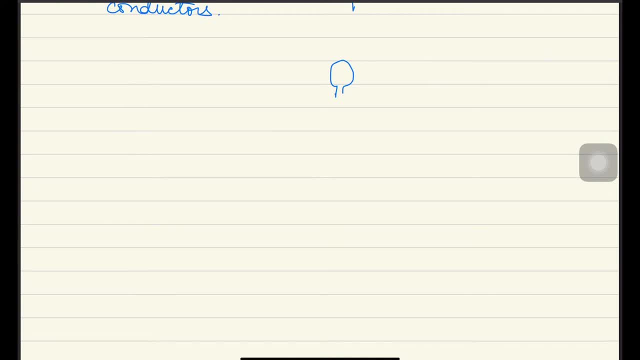 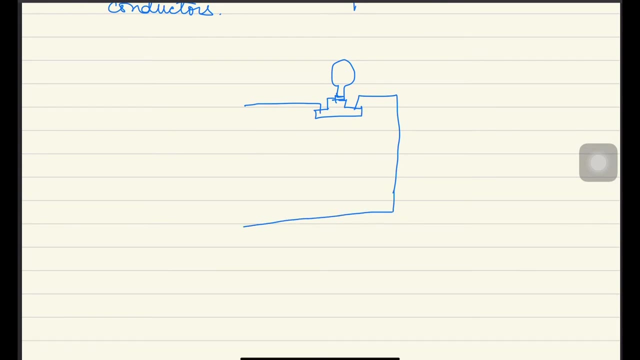 bulb. all right, i hope one point where you won't mind my drawing. okay, so this is the bulb. it is connected with a battery. okay, so the battery is here. that's the positive terminal. that's the negative terminal. positive terminal, negative terminal. it's connected with the battery- negative. 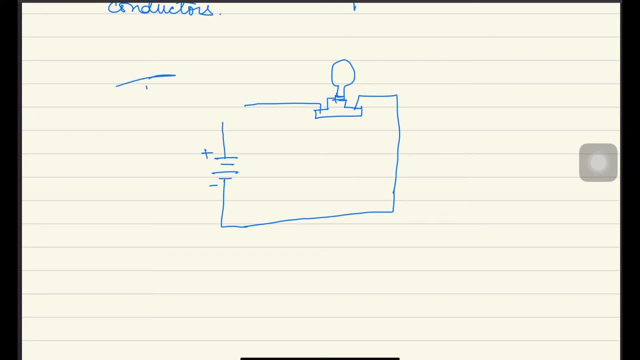 terminal, positive terminal. now i'll leave some space over here. so let's suppose i have this is my conductor and this object is my insulator. so first of all i'll attach my conductor and check what happens. okay, i'll place my conductor over here. this is my conductor. 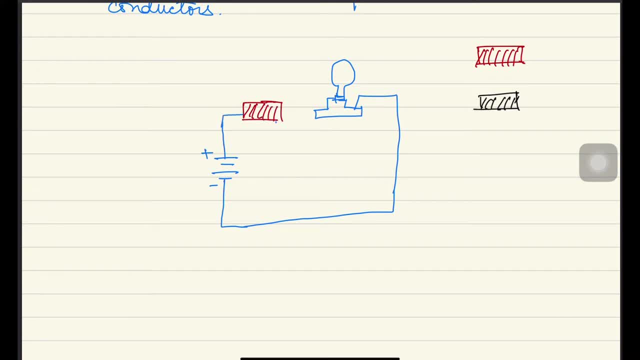 i'll connect this conductor with a wire from one end and the other wire from another end, and in this case the bulb will glow. the bulb will glow, okay, so from here i have seen that the current is being passed through this conductor, so the bulb is glowing. so it means this is the conductor. now i have to check the insulator. 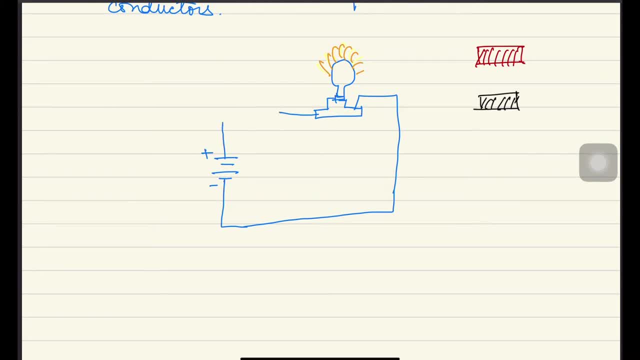 so i'll remove it and i'll attach that insulator. all right, so i'll attach this insulator. now what will happen? the ball will not glow, which means the current is not being passed through this insulator. simple, it's that much. simple. which means this object is an insulator because the current is not being passed through it and the 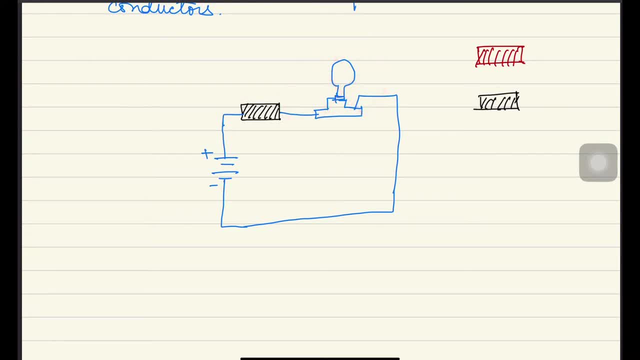 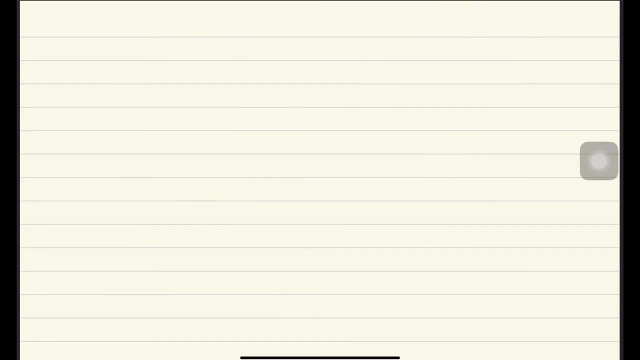 bulb is not glowing is not glowing. so that's how we'll just design a simple experiment to accent, to differentiate between an object, whether it's a conductor or insulator. okay, so that was the introductory part of topic 4.2. so now you have to discuss about the 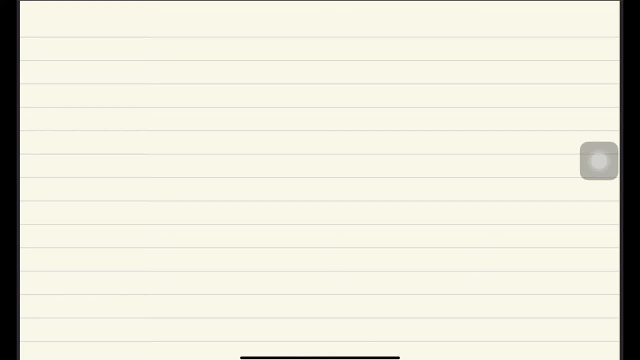 concept of electrical current. so that is exactly topic 4.2, point 2, and it's about the electrical current. so we'll discuss its definition first of all and then we'll discuss its unit direction and everything related to it. so, electric current, if you define the electric current, electric current is: 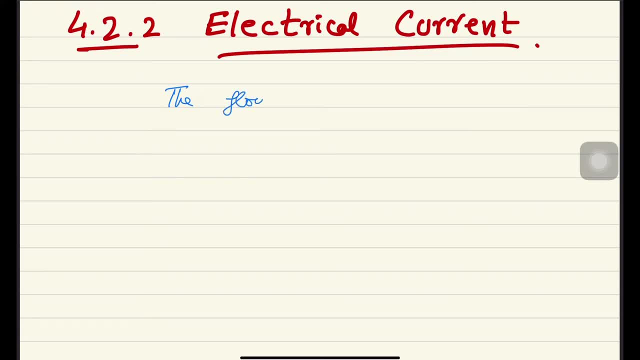 basically, it is the flow of charges per unit time. the flow of charges per unit time is called electrical, is called electric current. how fast the charges are flowing through any object in one second is defined, defines its elections, defines the electric current, for example. okay, I'll just write down the formula for for: 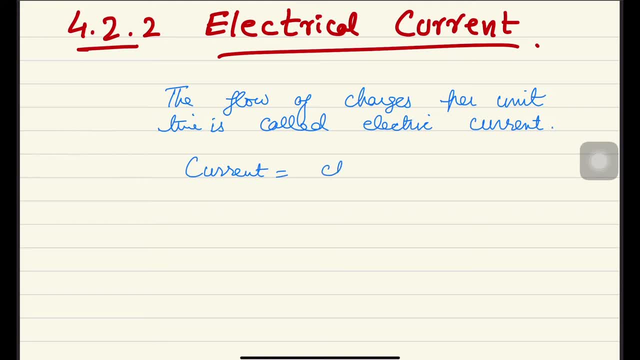 you. so electric current is equal to the charge divided by the time, and the unit of the electric current is ampere, represented with capital A. the unit of charge is coulomb. we represent it with capital C and the unit of time will be seconds and it is represented with S. okay, and the symbol that we use for 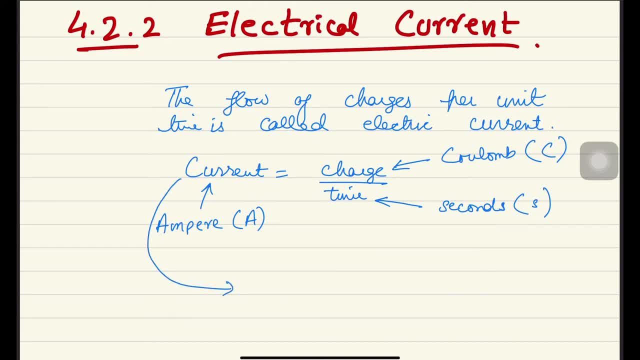 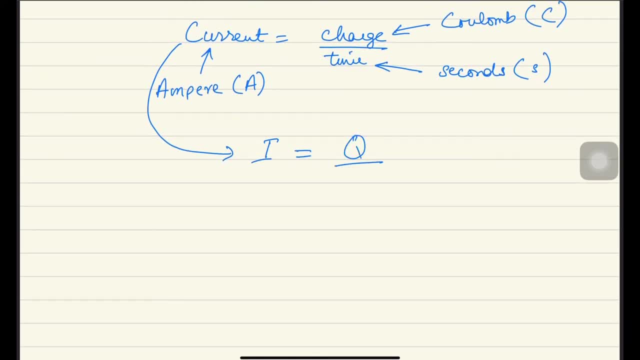 current is I, so it'll be like I equals to Q over T. Q is the symbol that is being used for the charge and T is the symbol that is used for the time. so electrical current is basically it is the flow of charges per unit time. how, the faster the charge. 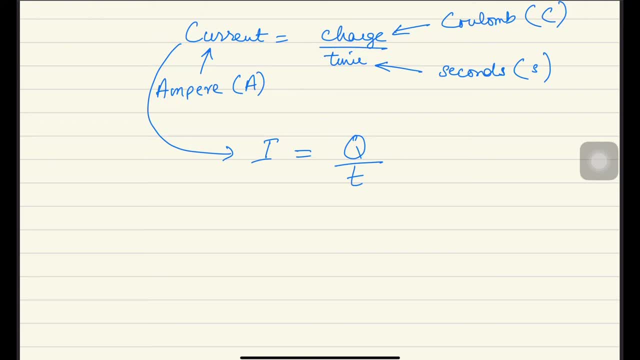 flows through an object, the more will be the current and the slower the charges will move through an object, the slower the lesser will be the current. but remember one thing: the electrical current can only pass through the conductor, the. it does not passes through the. it does not pass through the. 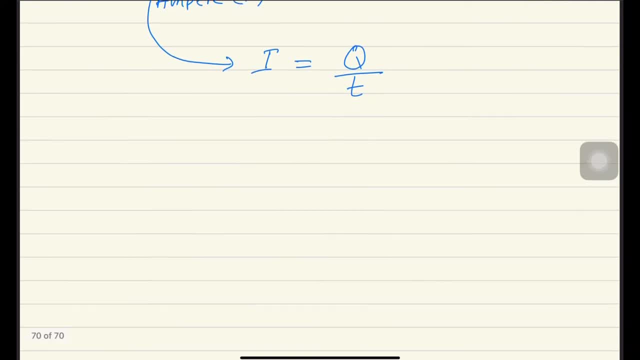 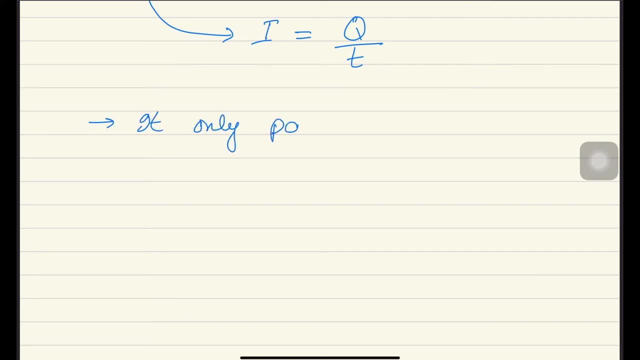 insulators. okay, so I'll write the point over here. it only passes through the conductors, like the metal objects, or you can say graphite as well- and it does not pass through the insulators. 3rd, 5th: Khan equal to 50 power felt Pow. 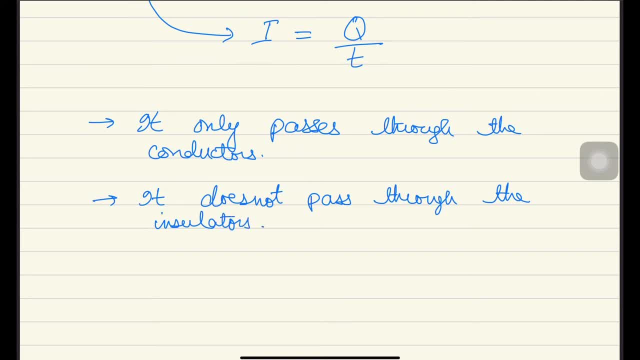 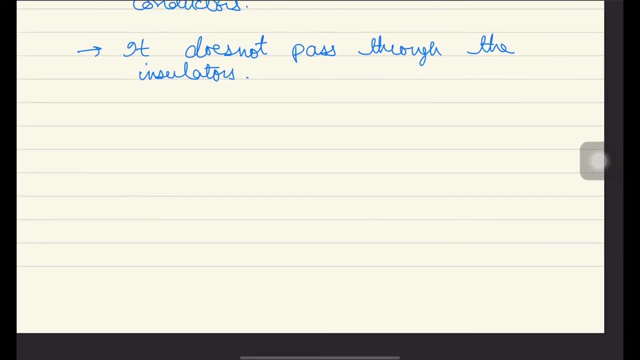 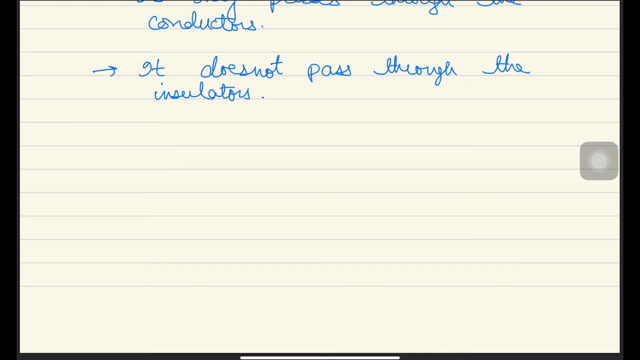 you have to keep that point. okay. now we have to discuss about the direction of current. remember I drew a figure before of a bullet and a battery that is connected to the world. so now, if you have to discuss the direction of the current and then we will discuss how can we measure the current, so let's suppose this is the battery. 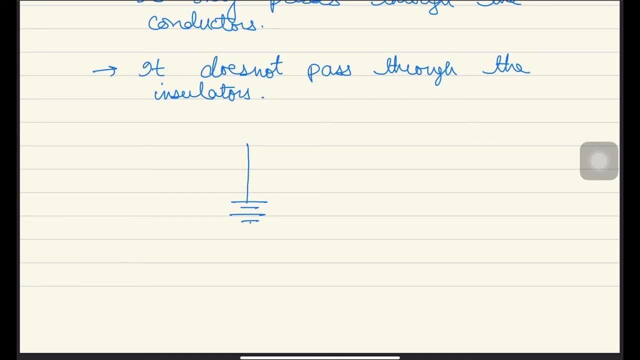 that's the positive terminal, negative terminal, positive terminal, negative terminal. and this battery is connected to a switch. this is the symbol of the switch, and then it is connected to a light bulb. so this is the symbol for the light bulb. i'm just using the symbols, i'm not. 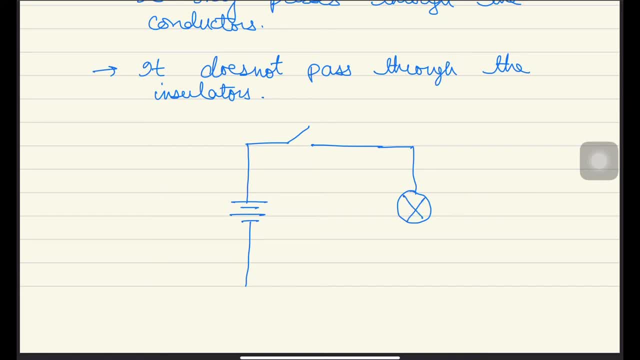 drawing the exact bulb. so this is the symbol for the light bulb. and there you go. these are. these are connected with the wires. so right now this switch is open, which means no current is being flown through the circuit. when we will close this switch, then what will happen? the current. 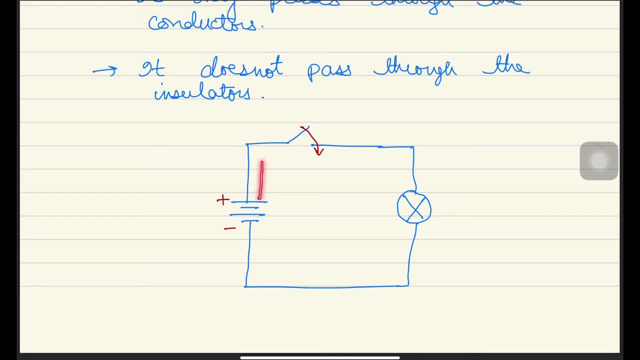 will start to flow from the positive terminal of the battery all the way through the bulb towards the negative terminal of the battery. so this will be the direction of the current that you have to keep in mind. the current always flows from the positive terminal of the battery towards the negative terminal of the. 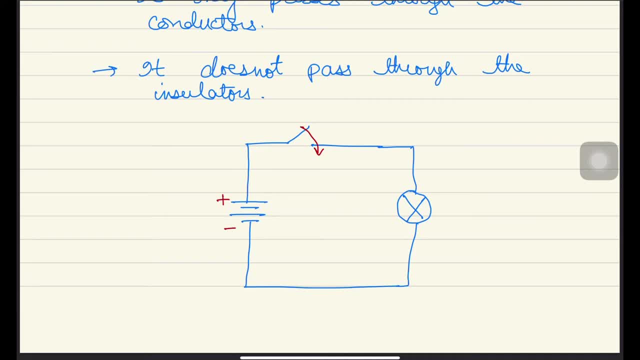 battery. i'll write it over here: um, it flows from the positive terminal of the battery towards the negative terminal of the battery towards the negative terminal. so that's the direction of the current. okay, now we have to discuss, um, okay, how the current flows. basically, so, the current flows due to the motion of electrons. okay, the current flows due. 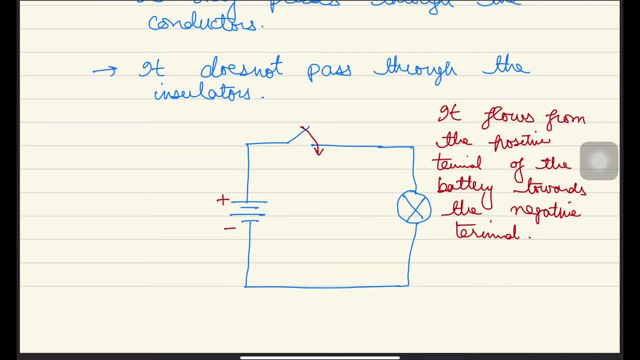 to the motion of electrons. but the question is: electrons are negatively charged, then how come they flow from the positive terminal towards the negative terminal? it's not like that. the electrons flow from the negative terminal because they are, they are repelled by this negative terminal, so the flow of electron is from the negative terminal of the battery. 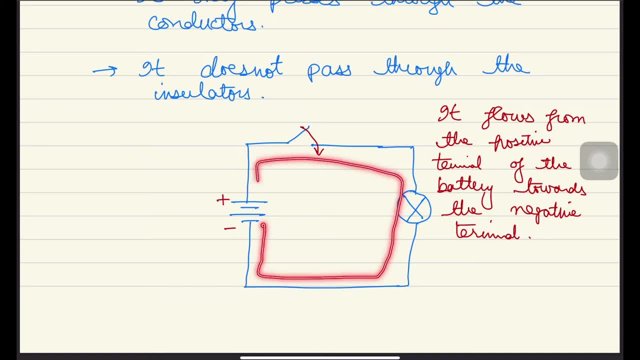 towards the positive terminal, like that. this is the flow of electron. but over here we are not discussing the flow of electrons, we are discussing the direction of the current. so the direction of current is opposite to the flow of electron. that is called the conventional current. before it was discovered that the current flows. 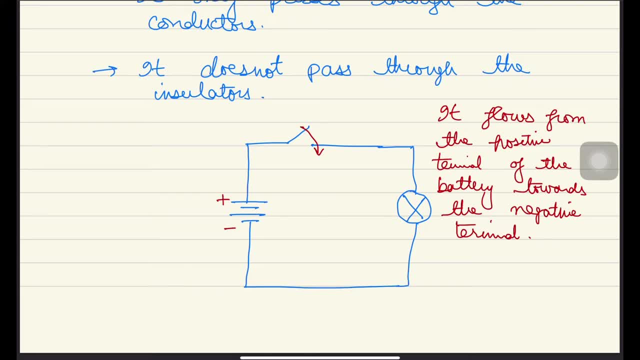 due to the electrons, everyone assumed that the current flows from the positive terminal of the battery towards the negative terminal of the battery, and when it was discovered that the current flows due to the flow of the electrons, then it did not change any outcomes. so the scientist kept the direction of the current from the positive terminal of the 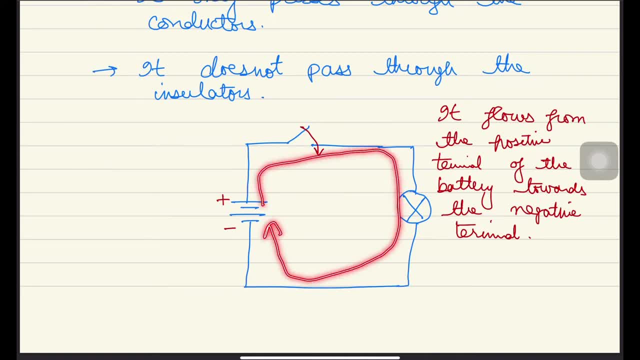 battery towards the negative terminal of the battery, because it does not make any difference. you have to keep in mind that the current always flows from the positive terminal of the battery towards the negative terminal of the battery period. now we have to discuss about the device that is used to measure the current. 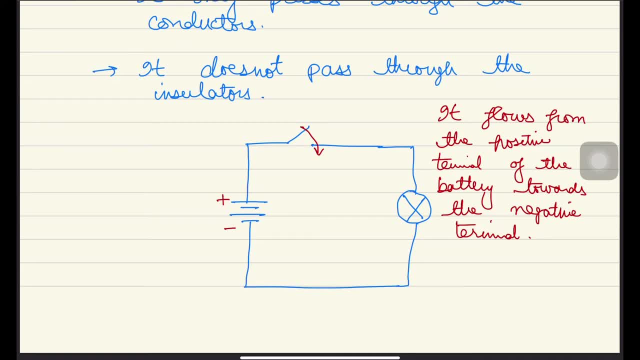 like: how can we measure the current? so the device that is used to measure the current is called ammeter. if i attach the ammeter in this circuit, i'll just draw a circle over here and write A for ammeter and I'll just connect it like that. so this is how they connect the ammeter and in the circuit and this: 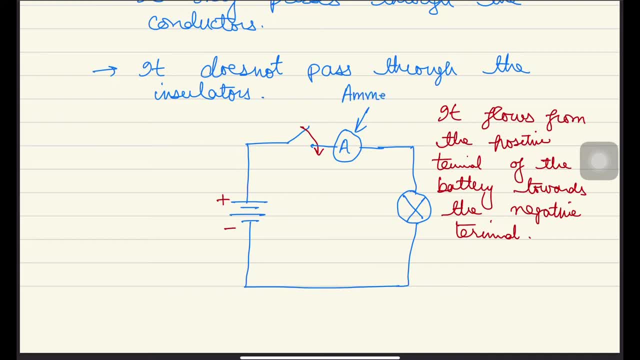 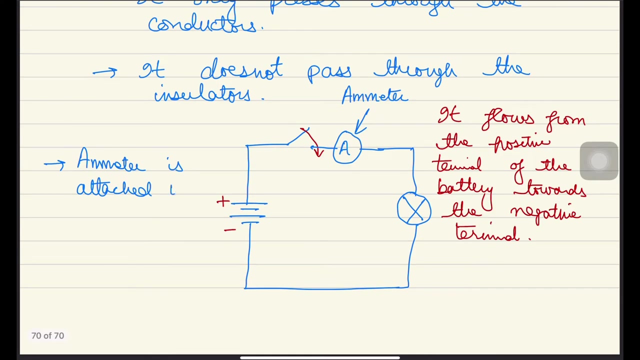 device is used to measure the electrical current. okay, so ammeter is attached in series. this is the series attachment. okay, that's the series attachment of ammeter. so ammeter is attached in series and it is used to measure the electric current. it is used to measure the electric current. 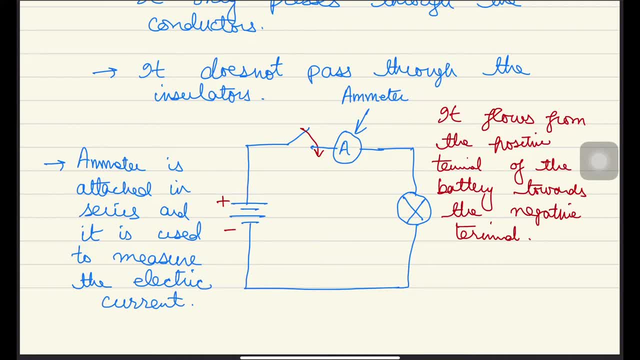 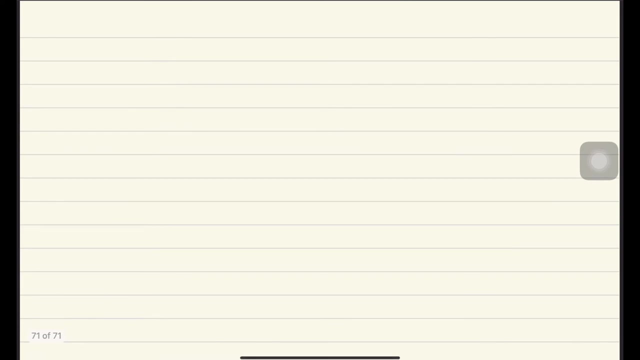 okay, so that's it about the electrical current, but I have to discuss two types of electric current as well. so you'll you'll discover that there you'll discuss, like in the later chapters, that that there are two types of electrical currents. so types of electrical current. 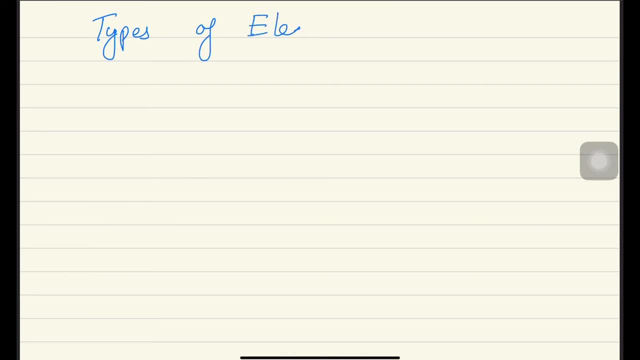 types of electrical currents. number one, I'll just write it over here: direct current. so this type of current is mainly produced by the batteries. all types of batteries: they produce the direct current, no matter it's the inverter battery or the mobile battery or the laptop battery, all type of batteries tip, they produce the. 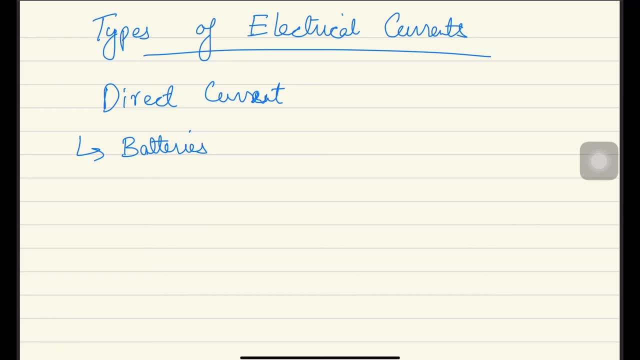 direct current and, up to some extent, the solar panels. they also produce the direct current and the other one is the alternating current. so in our homes we receive the alternating current, and usually the source of alternating current are the generators. so any generator, no matter it's at the power plant, it's at the like, it's a wind. 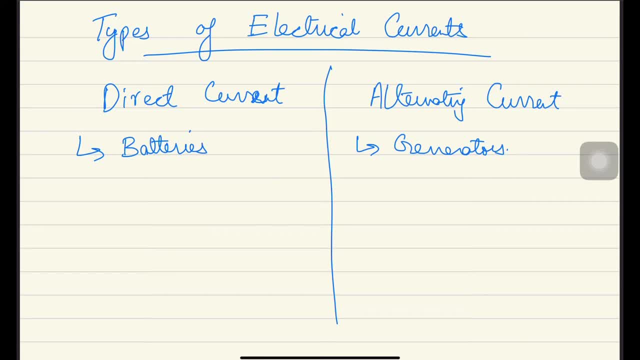 turbine, it's hydropower plant, or you can say its the plant by the, by the waves, or the normal engine, like the normal generator, like fuel-based generative, all type of generators. they produce the alternating current and in our household we also use the alternating current because alternating current is best for the motors and you know like. 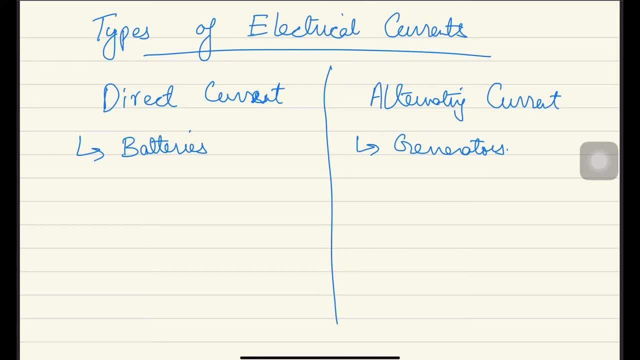 the motors are everywhere. the motors like water, motor oil or secondary motor or a solid её chromosomes can pop up everywhere. the iguags and water watervari Lautenburgs motor in the fans in the air conditioner, like the motors, are everywhere. so alternating current is. 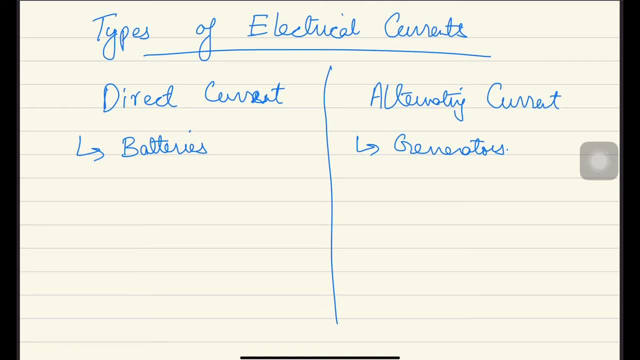 the best suitable for the motors and also it is easy to transfer from one point to another as compared to the direct current. so in our household we use alternating current and for our portable devices normally we use the direct current. so these are the two types of currents that you. 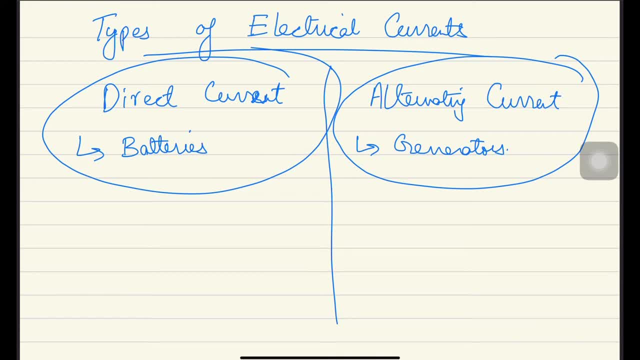 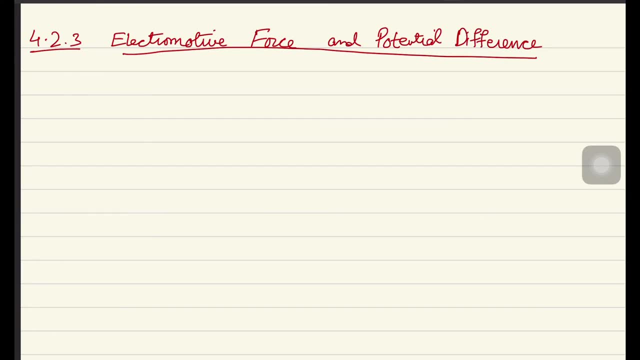 should know- and this is it about the topic- from the electric current. all right, so now we have to discuss about the electromotive force and the potential difference. so electromotive force and the potential difference, they are basically almost same with a slight difference. so in this topic, 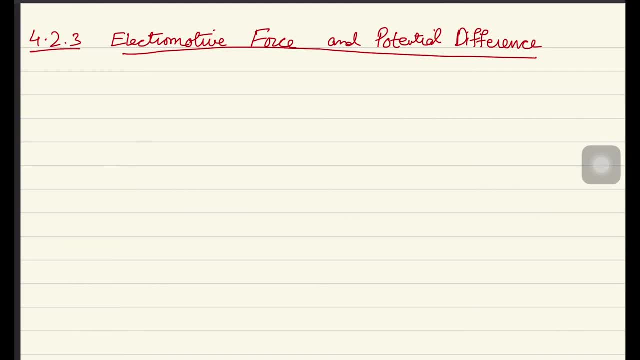 we'll, first of all, we'll discuss about that difference, okay, so for that purpose i have to draw an electrical circuit. so here's the battery. it's connected with the light bulb. that's the light bulb. okay, so that's the negative terminal of the battery. that's the positive terminal of the battery. 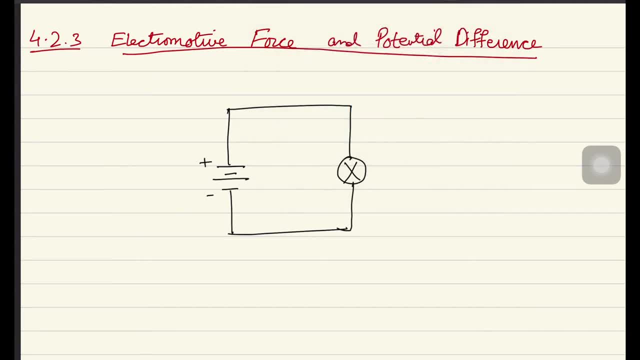 now there's a charge that's gonna flow from the post, as i told you that the current flows from the positive terminal of the battery towards the negative terminal of the battery. okay, um, in fact, let me just draw two bulbs so it'll be more clear to you. 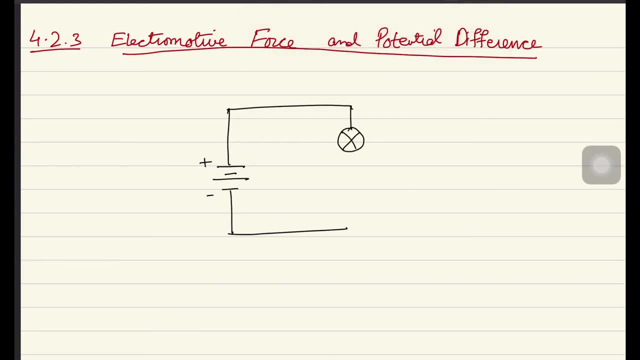 all right. so that's one bulb bulb, number one. here's another bulb, bulb, number two- and the charge flows from the positive terminal of the battery towards all the way towards the negative terminal of the battery. now, first of all, we will define the electromotive force. so electromotive force is basically, it is the amount of work done. 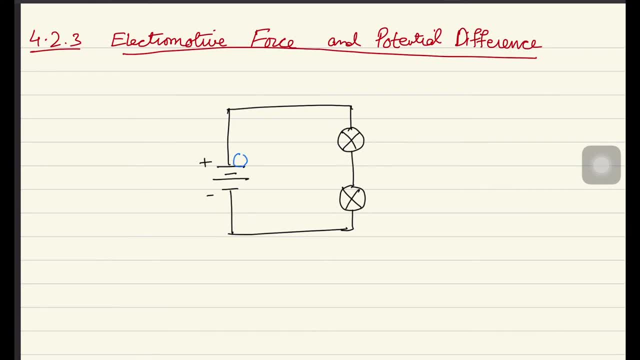 that we do on a charge. let's suppose one charge is starting from this position and it is moving all the way through the circuit. okay, i repeat, one charge is starting from this positive terminal of the battery and it is moving all the way through bulb number one and bulb number two and reaches the negative terminal. 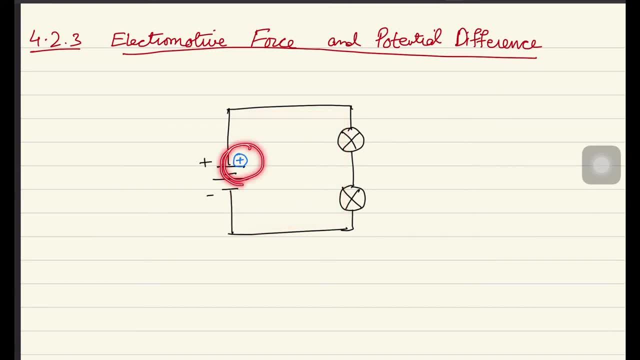 so the work done that has been done on this positive charge is called the electromotive force. got it. now i'll write down its definition: the amount of work done, the amount of work done on a charge, on a charge in order to move it throughout the circuit. 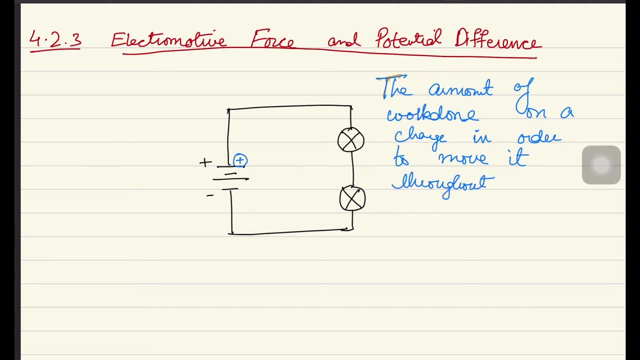 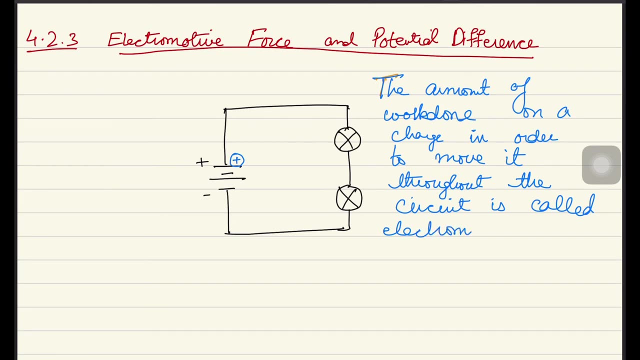 throughout the circuit is called emf, or we can say electromotive force. it's called electromotive force, okay. or emf as a short version. the unit of the formula for the emf is- i'll write it over here: emf is equal to work done. 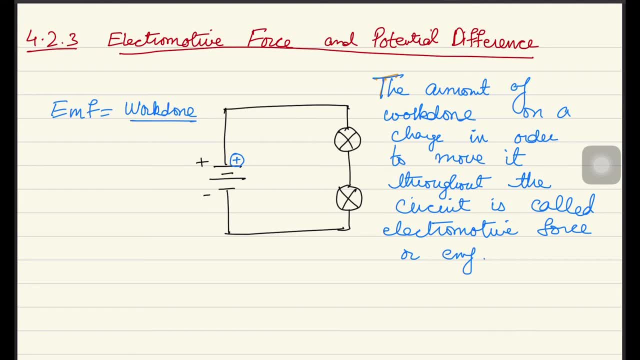 since it's work done per unit charge, so you can see that it's working on a charge. i'll say work done divided by the charge and symbolically we can write: we represent emf with v, we represent charge with worked on with w and charge with q. 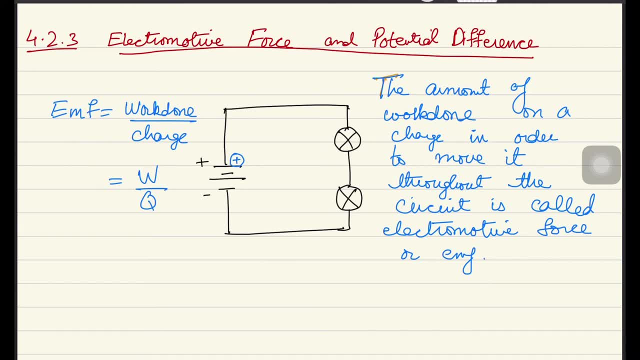 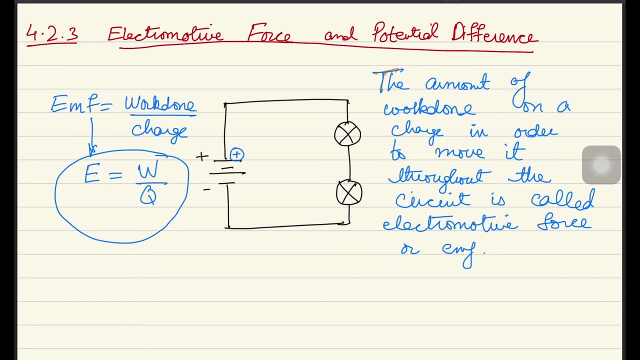 so it'll be like. in fact, we represent emf with e. it's not energy, its emf okay. so emf is equal to work done per unit charge. or we can say e is equal to w over q. now if we talk about the unit of the emf, 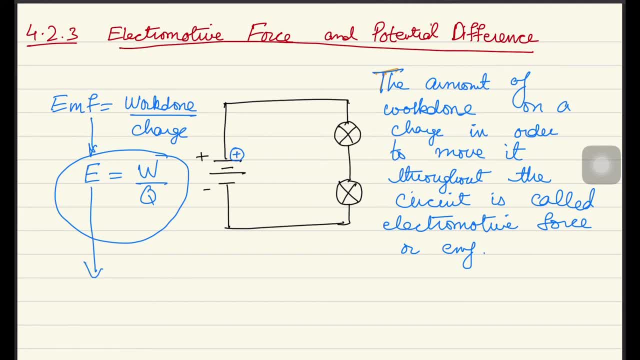 the unit of the emf is volt and represent volt with capital V. okay, now volt is basically equal to, if we discuss the volt in in terms of SI units. so volt itself is equal to joule per coulomb. okay, why? because the unit of work done is joule and the unit of 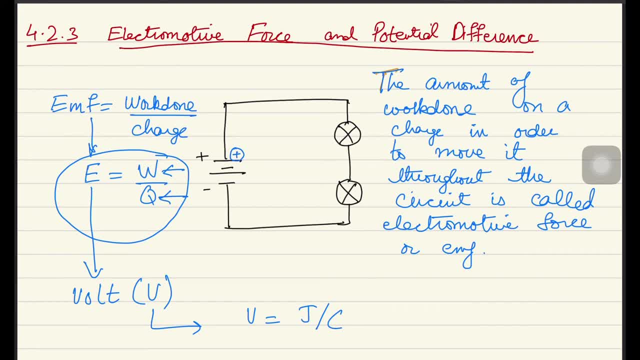 charge is coulomb. so we have, we can discover, we can define the EMF with two units. one is the volt and the other one is joule per coulomb j over C. okay, but the main idea that you have to keep in mind about the concept of EMF is the 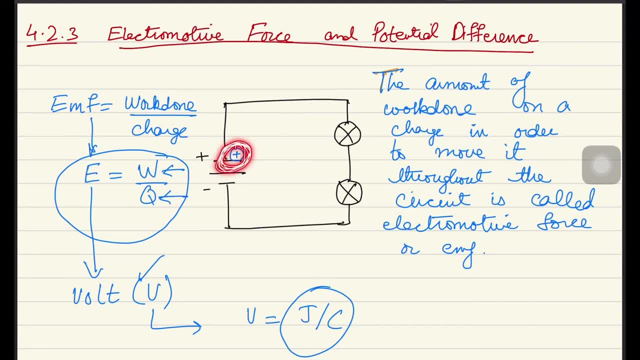 amount of work done that will be done on this particular charge in order to move it to the high current throughout this whole circuit. okay, that is called the work done. that is called the emf. now the next thing, and quite similar thing that we have to discuss is about the 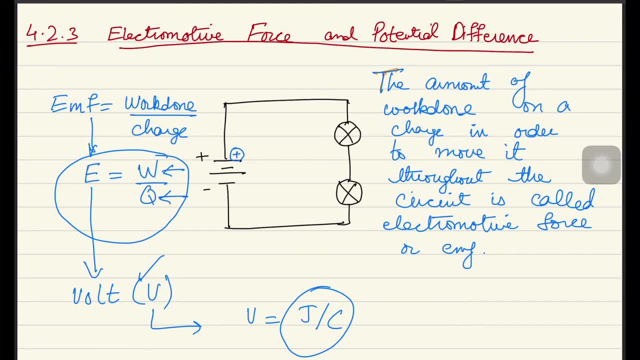 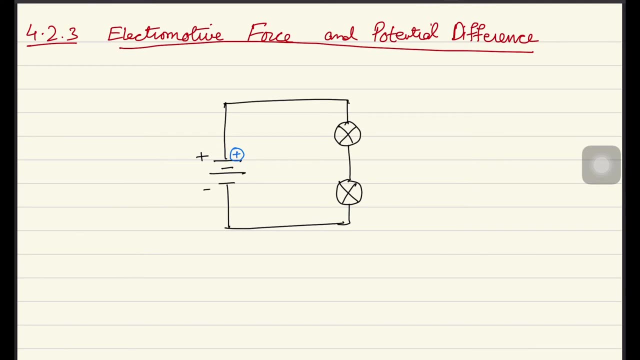 potential difference. there's a slight difference between the emf and the potential difference, so for that purpose, i have to erase it all. i accept this circuit. okay. now, in order to understand the potential difference, i'll resume my story from here now. look, this is the charge. it is starting. 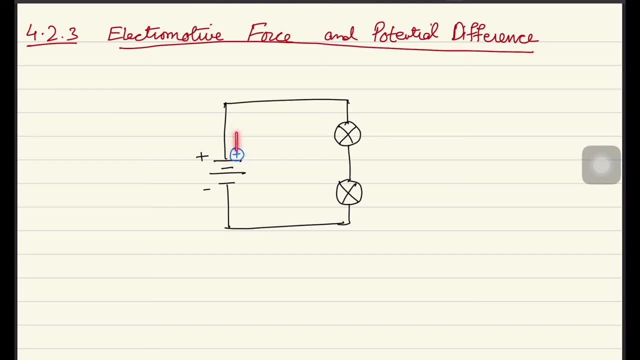 from the positive terminal of the battery. it started from here and moved at this particular point, at this point, okay. and now, after some time, it moved from this point to this point, okay. so this positive charge has moved through the bulb number one. so the amount of work done that we have to apply on this positive 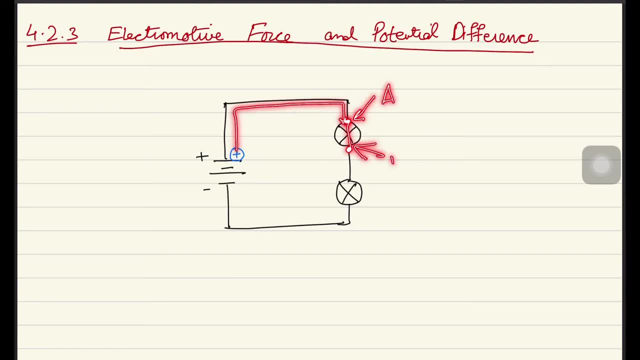 charge in order to move from. let's suppose this is a position a and that is position b. okay, so the amount of work done that we have to do in on this positive charge in order to move from position a towards position, towards position b is called the potential difference. 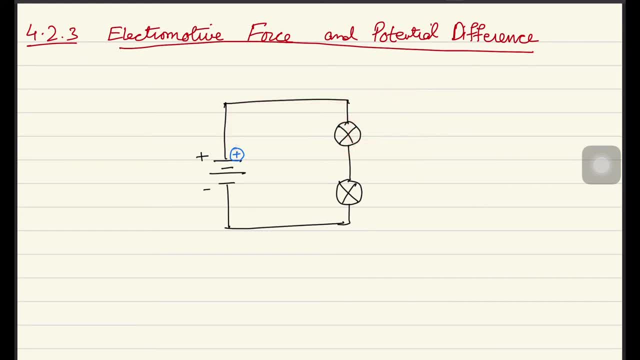 okay, now, after some time that charged moved over here from this position to this one. and now the amount of work then that we have to do on to this charge in order to move from this position a towards to this position b. that is called the potential difference across bulb number two. okay, so that's the difference between the emf and the potential. 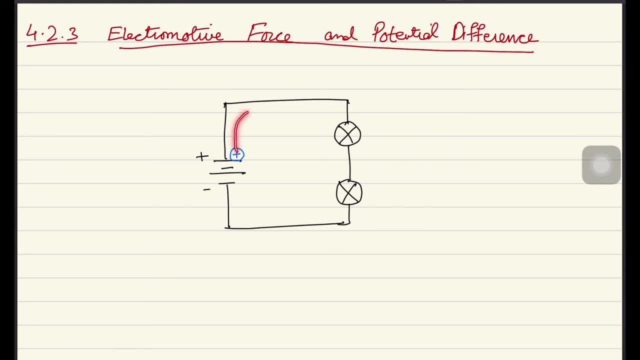 difference. emf is means the work done in order to move the charge throughout the circuit on the charge, just to move it through one electrical component, one electrical component. so that's the difference between the um, emf and the potential difference. now i'm going to write down the definition formula and everything so that you can note it down. okay, the amount of 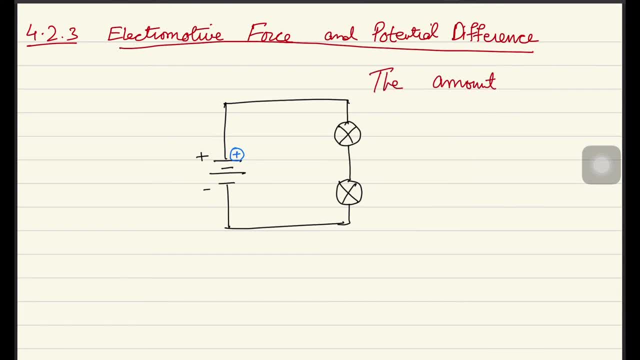 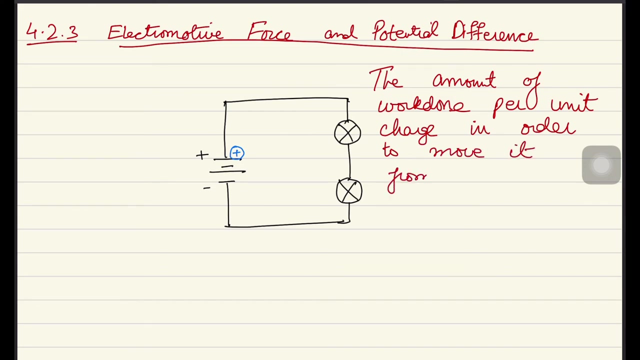 work done: the amount of work done per unit charge in order to move it from one point to another, to another, across a, across an electrical component. in this case, this bulb was electrical component across an electrical component. so that amount of work done on electric charge in order to move from one point to another. 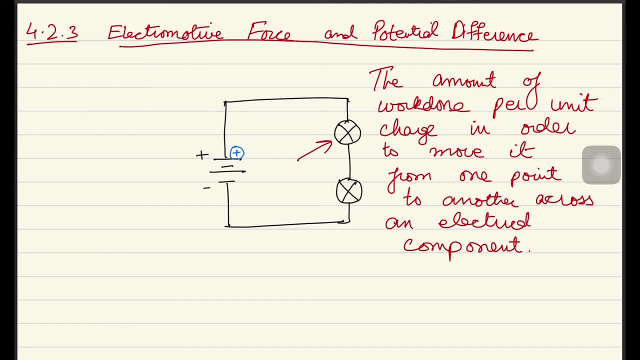 is called the potential difference and we can write it as pd equals to vd, work done divided by the charge, or we can we represent potential difference with v, so it'll be like v equals to w over q and the unit. of course the unit we have like two units. one is volt, that is most commonly used and 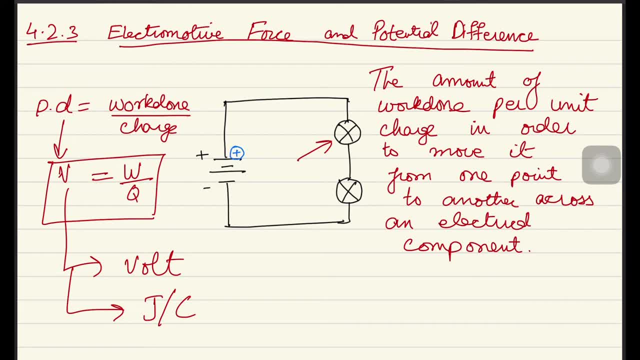 the other one is joule per coulomb. like everything else is same. the only difference is in the definition of the potential difference and the electromotive force. okay, now we have to discuss about the device, about the, yeah, about the instrument that is used to measure this potential difference. 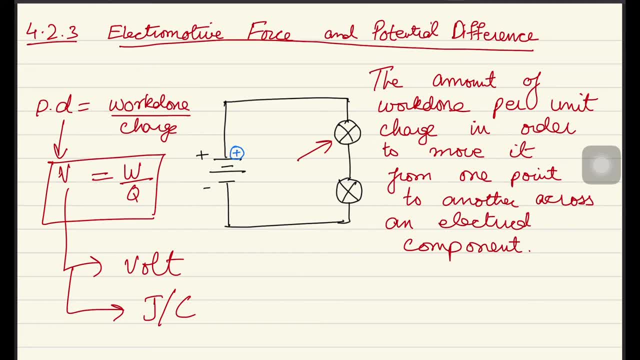 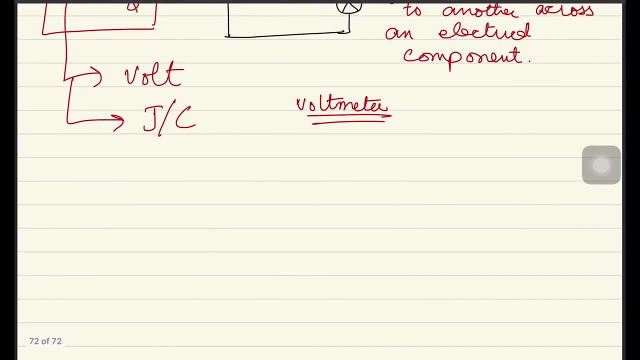 so the instrument that is used to measure this, to which is used to make the potential difference across any object, is called the voltmeter. okay, so now we have to discuss about the voltmeter. so voltmeter is basically, it is the component, it is the instrument, basically the 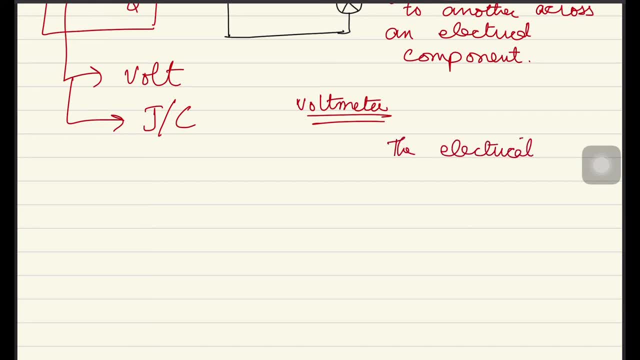 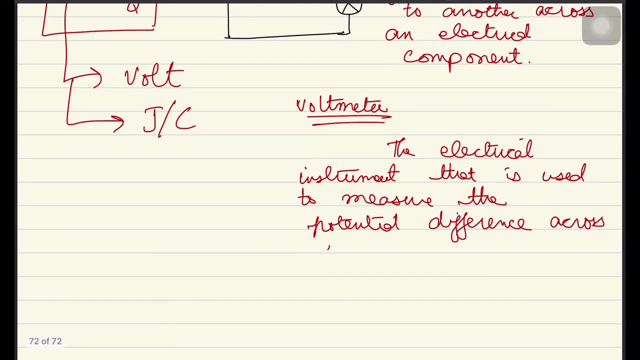 electrical instrument that is used to measure the potential difference, to measure, use, to merge the potential difference across an object, across an object. so that's the role of voltmeter and, about the like, how we can attach the voltmeter in a circuit. so basically, we attach the voltmeter in parallel. 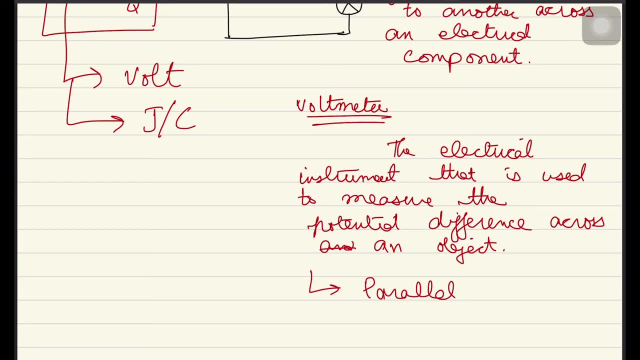 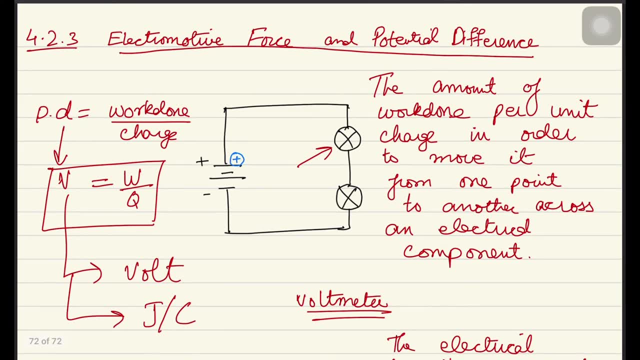 so it is attached in parallel points in an electrical circuit. so we are trying to position it. so it ist circuit to measure the potential difference or the voltage. voltage is another word for the potential difference. we call it potential difference or the voltage. so potential difference and voltage are same voltage. 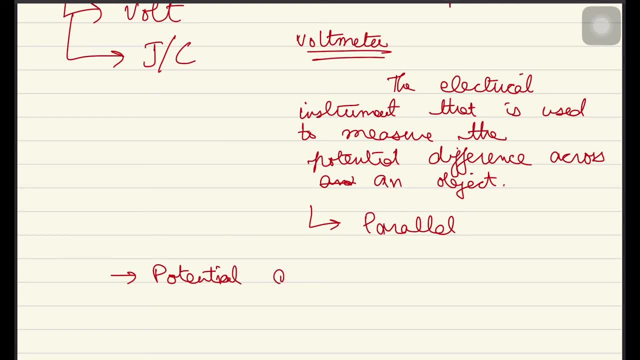 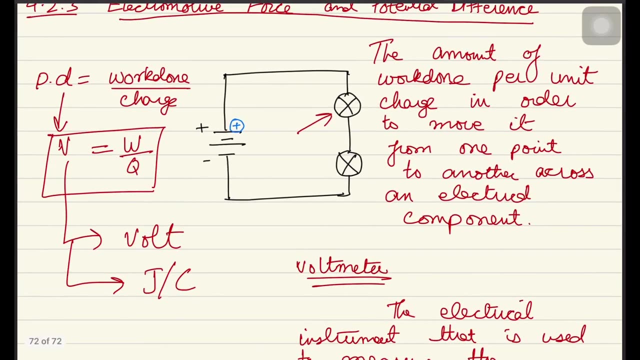 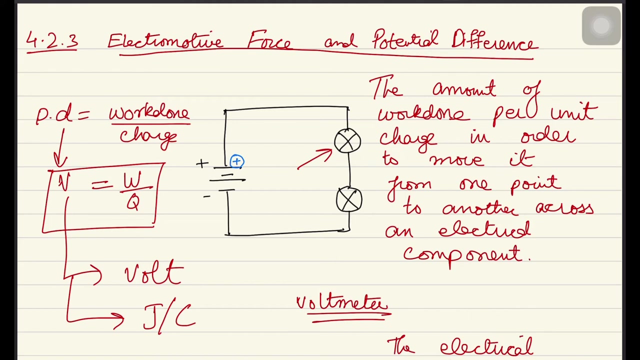 is just another word for potential difference. so potential difference is same as voltage. okay, now we have to check. we have to see how we can attach a voltmeter in an electrical circuit to measure its voltage or the potential difference. so let me just remove this definition now. I'll write it over here. 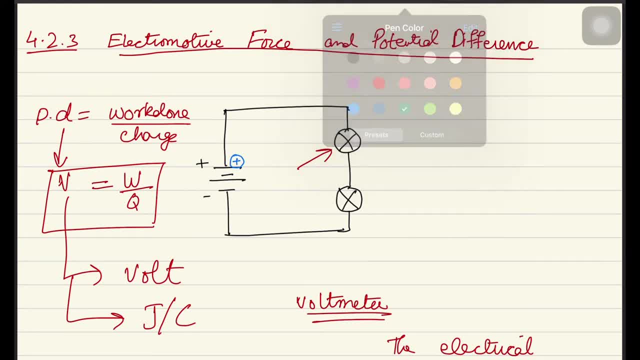 so we attach the wattmeter in parallel. so this, that's the bell commission, that's the voltmeter I represented with V. there you go. so that's how we attach the voltmeter with the bulb so that we can measure its potential difference. now the next thing that you have to discuss is the EMF, or the voltage in a parallel. 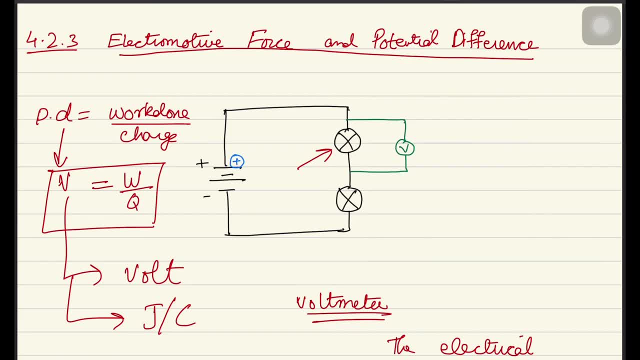 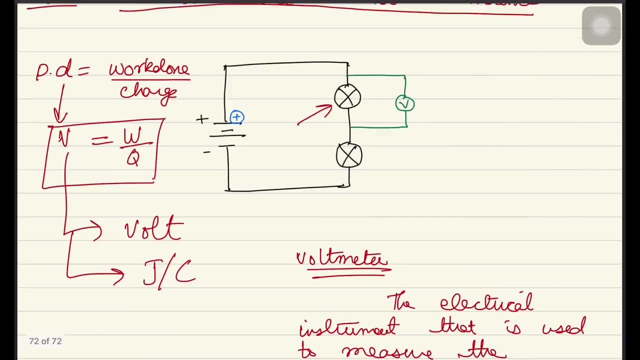 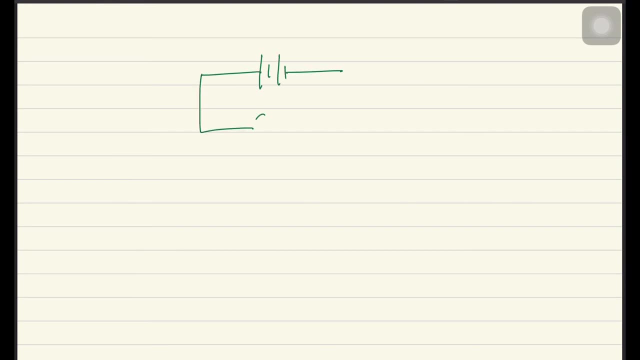 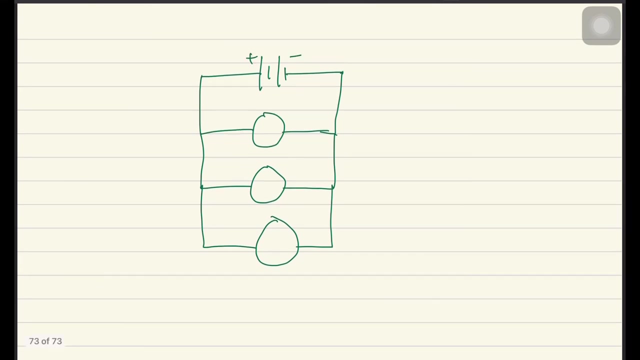 circuit, Oh circuit. or you can say: okay, let me, let me just draw a parallel circuit so you can understand it properly. so, for example, this is the battery, this is belt number one, that's belt number two, that's belt number three. the voltage of this battery, or the potential difference of this battery, is 12 volts, that's. 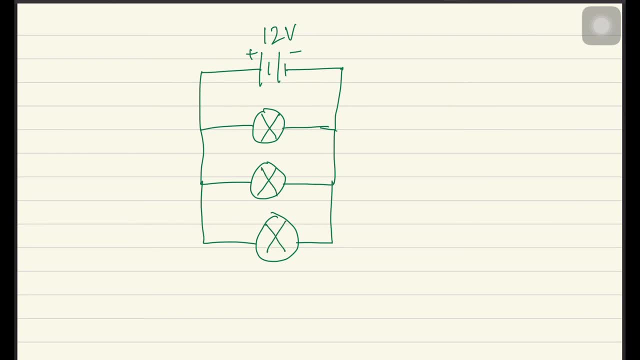 belt number one, belt number two, belt number three. now the voltage, or the potential difference across this bulk. well, number one, well, number two and belt number three will be same, and that voltage will be equal to 12 volts, which means, well, number one will have 12 volts across it. well, number two will have 12. 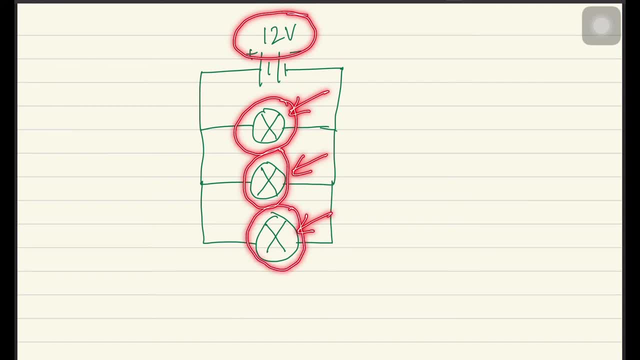 volts across it. and well, number three will have 12 volts across it, so we can say that the potential difference or the voltage, the voltage or potential difference remains same in series. and so in parallel- sorry pardon, in parallel, this is the parallel combination. okay, now let's draw a series. 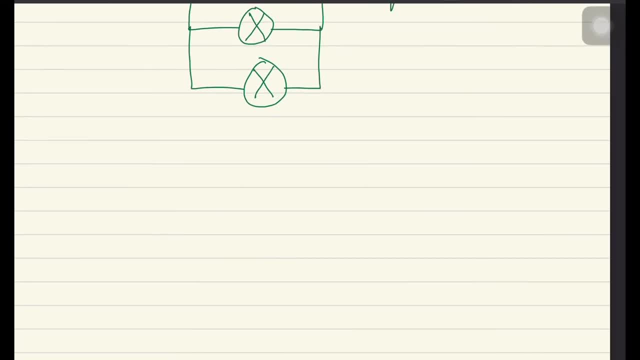 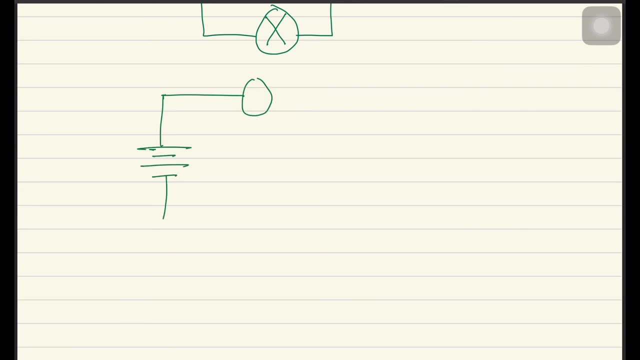 combination as well. so for the series combination, let's suppose we have this battery, this is well number one, well number two and well number three. now one, two and three negative terminal, positive terminal, this batteries of 12 volts. now this is the series combination, this is the series combination in the series. 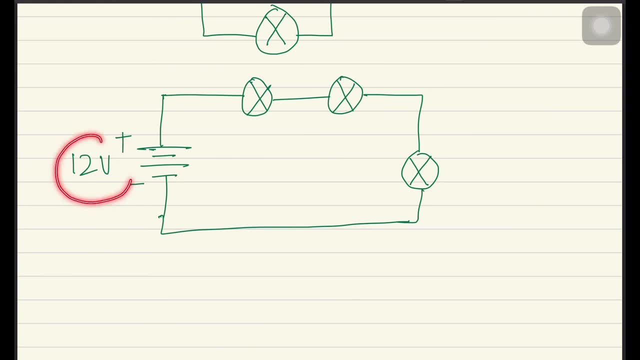 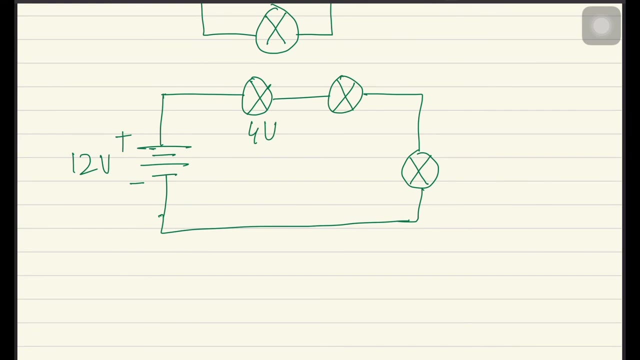 combination. this 12 volts will be divided among bulb number 1, bulb number 2, and bulb number 3.. So 4 volts will be given to bulb number 1,, 4 volts will be given to bulb number 2, and. 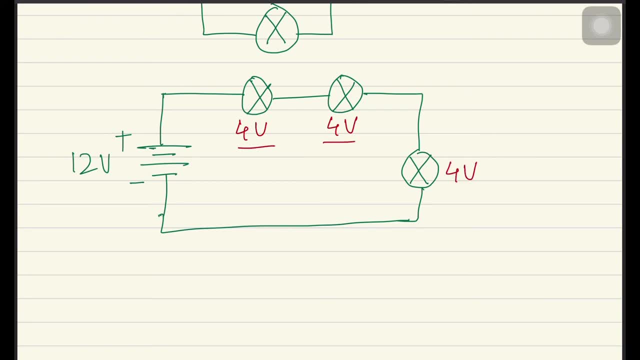 4 volts will be given to bulb number 3.. So when you add all of these voltages, they sum up to 12 volts. So that's how you'll work it out. that's how you'll see the voltage or the potential difference. 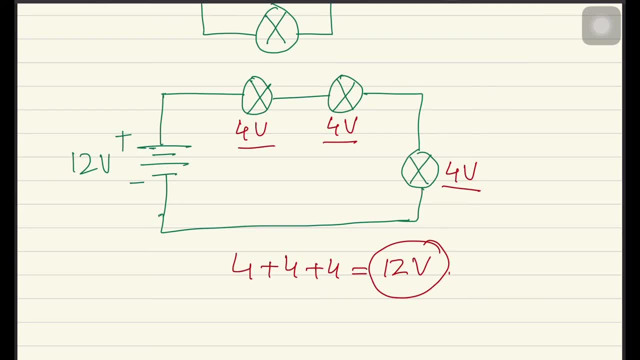 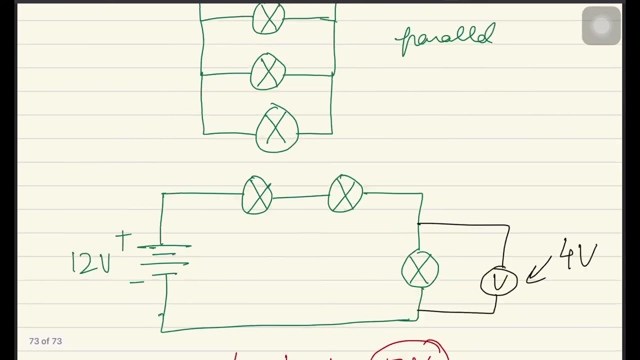 in parallel and the series combination. And let's discuss it a bit further, For example, within the same circuit. if you attach a voltmeter, for example, let's suppose I attach a voltmeter across this bulb, So this voltmeter will show me 4 volts. 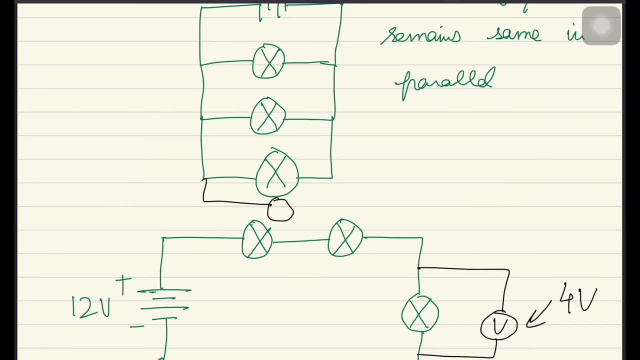 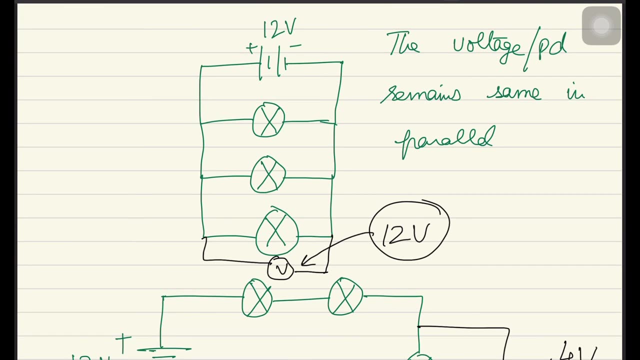 And if I attach the voltmeter over here, then this voltmeter will show me 12 volts. So voltmeter is just a device that is used to measure the potential difference across our electrical components. Okay, so yeah, this is it about the electromotive force, potential difference and the characteristics. 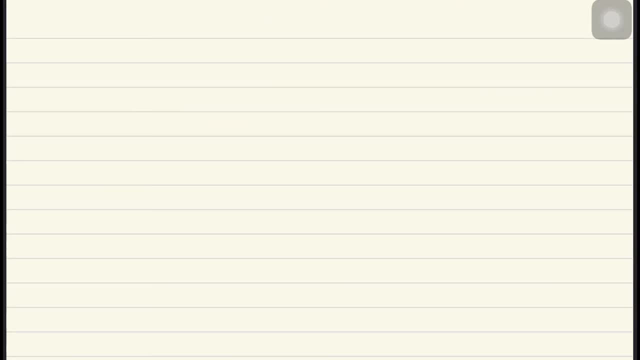 of the potential difference or the voltage in series and parallel combination. Okay, so now we have to discuss the last subtopic of this topic, and that is about the resistance. What is a resistance? So resistance is simply a resistance, a resistance. 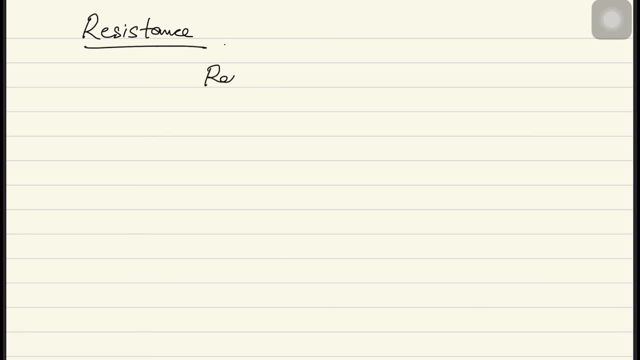 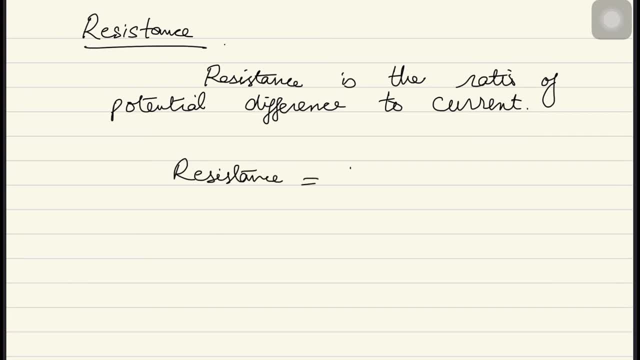 potential difference. i'll just write it as pd over current. that is simply the resistance and symbolically, if i write it, it will be like r equals to v over i, where v is the symbol for the potential difference, i is the symbol for the current and r is the symbol for the resistance. 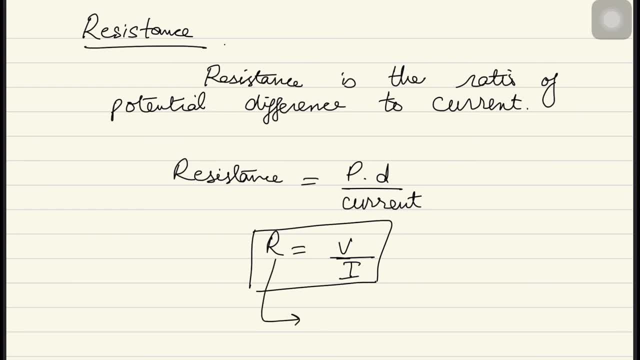 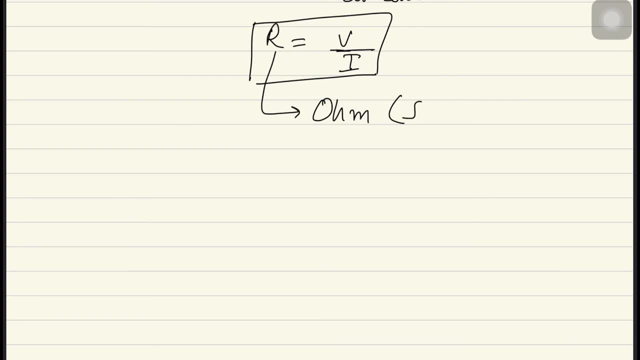 as far as the units are concerned. so the units of resistance are ohm, ohm, and this is the symbol of the unit of resistance. okay, and now we have to. we have to design an experiment by which we will the resistance of an object. okay, so what we will do is i will draw an electrical circuit. 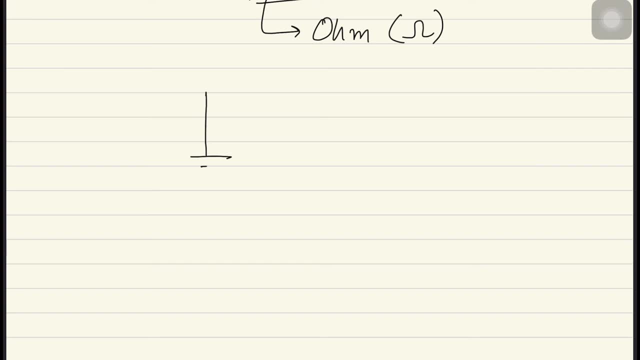 an electrical circuit. this is the battery, and i will put a variable resistor. i'll let you know what. what will it do? then? i'll put an ammeter and the voltmeter- sorry, the bulb, light bulb- and this will be connected with the negative terminal of the battery and across it. 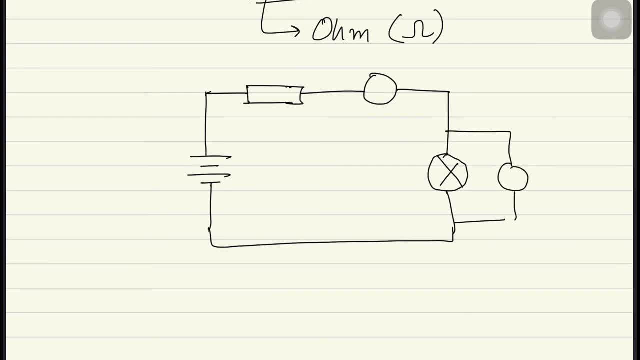 i will attach a voltmeter like that. that's the ammeter, this is the voltmeter and this is the variable resistor. this is the positive terminal of the battery. that's the negative terminal of the battery. now i will change. i will keep this variable resistor to be maximum. so minimum current. 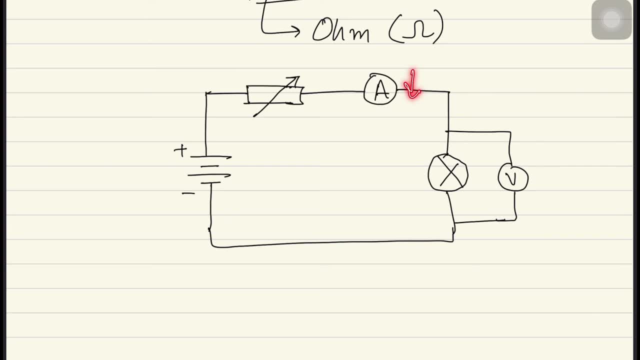 will pass through this circuit and after that i will check the voltage across the light bulb and then after some time i'll decrease this resistance so more current will pass. then i'll decrease it further. more current will pass, decrease it further, more can pass, and in the end i'll note: 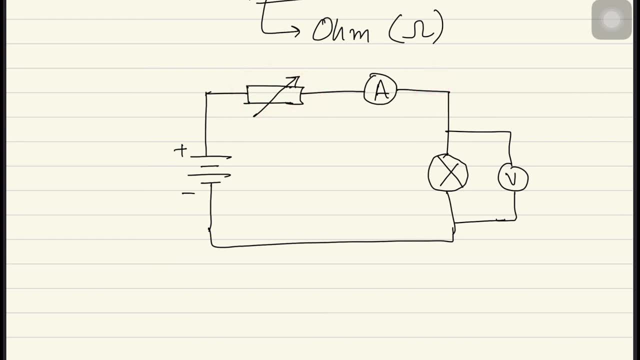 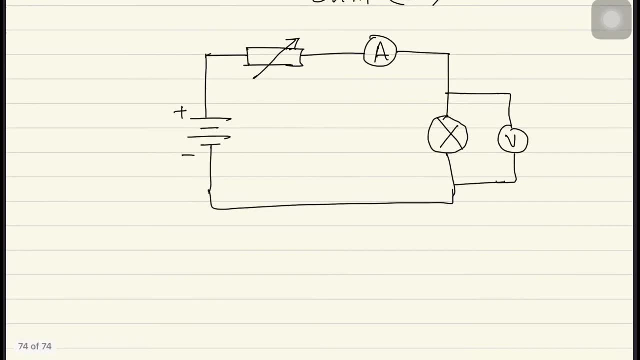 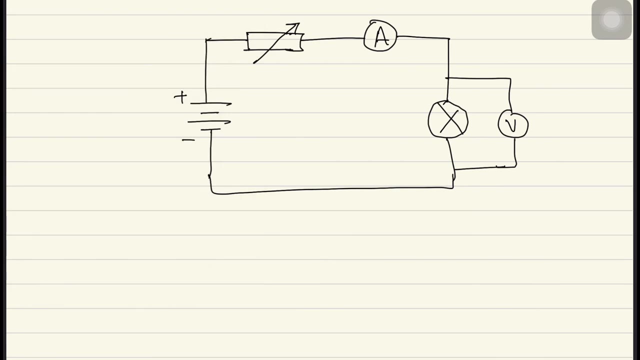 down all the readings of the current and the voltages and from there i'll work out the resistance of this light bulb, how i'll show you. so what i'll do is i will make a graph over here, i'll draw a graph over here where i'll have the current in the x-axis and i will have the voltage in the y-axis. 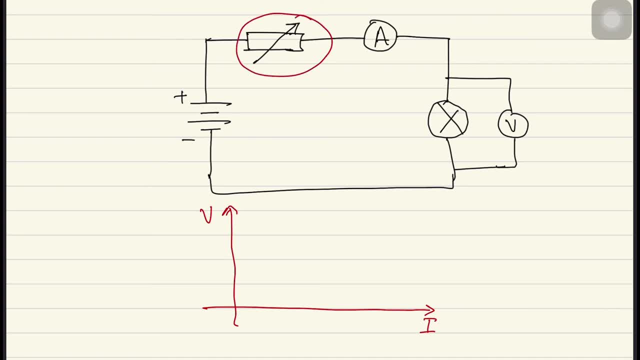 okay, i'll keep this variable resistor to the max so i'll have minimum current. let's put over here: so i have zero current and zero voltage. i'll decrease, I'll decrease this resistance so the current could increase through this ammeter And when the current increases, the voltage will increase as well. 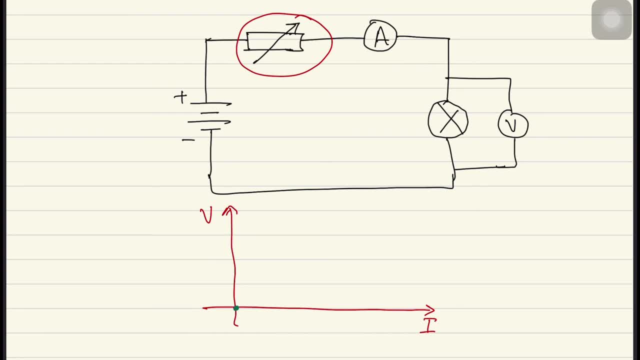 So when the current increases, the voltage increases, and I'll get my new position over here, then over here, then over here, then over here, and then over here. So I'll just draw a straight line that joins all the points and then I'll find out the 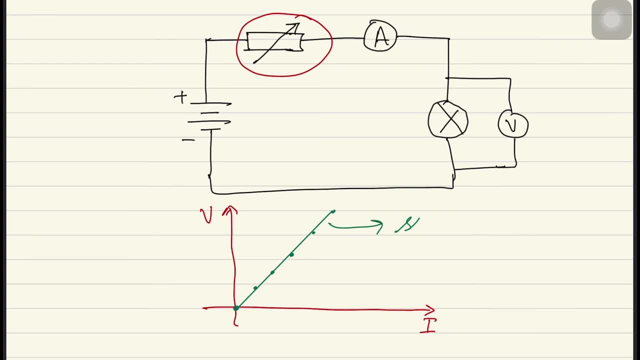 slope of this straight line. Slope means how much is the rise in this line and how much is the run in this line. So slope is simply rise over run. For example, the voltage increased from 0 volts to 20 volts, so the rise will be 20.. 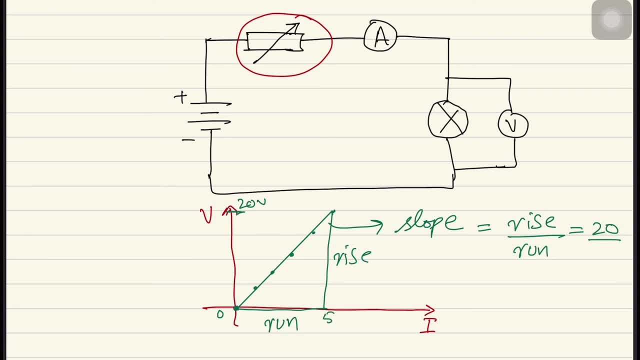 And the current increases from 0 ampere to, for example, 5 ampere. so the run will be 5.. When I will divide them, I will get 4.. So 4 is the slope which will give me the resistance. 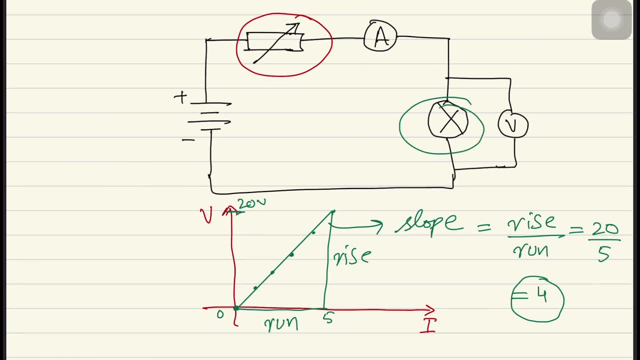 So the resistance of this light bulb is 4 ohms. Did you get it? So by this experiment we will find out the resistance of this light bulb. Now there's a twist, And the twist is in this experiment we did not consider the increase in temperature with. 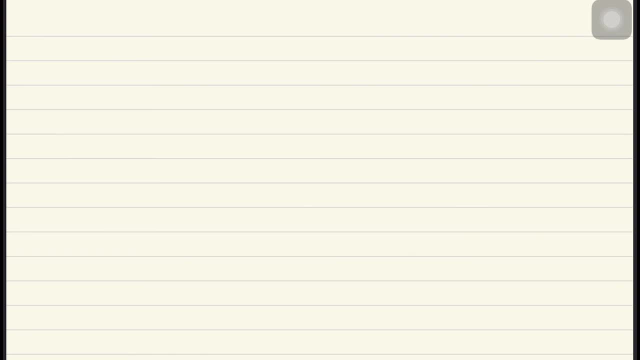 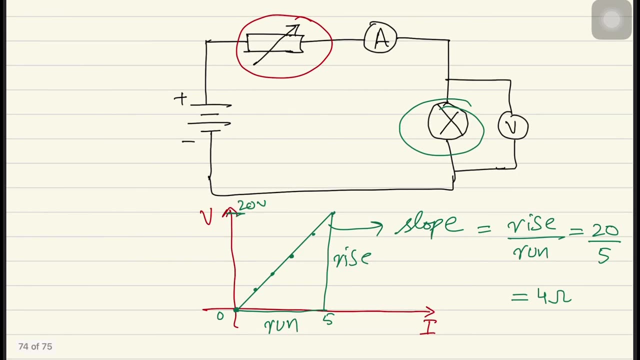 the increase in current. So let's come back onto it. When you increase the current, the voltage will increase across the bulb And, of course, the current will also increase across the bulb. So when the current increases across the bulb, it will increase the temperature of the bulb. 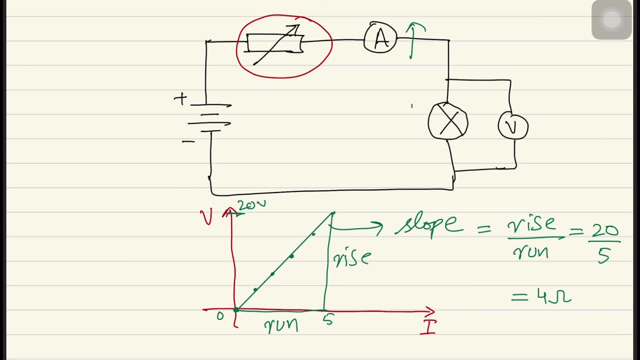 So when the temperature of the bulb will increase, its resistance will increase. That will cause to decrease the current. So in actual, our graph will not be our graph for this light bulb will not be a straight line. It will be a curved graph. 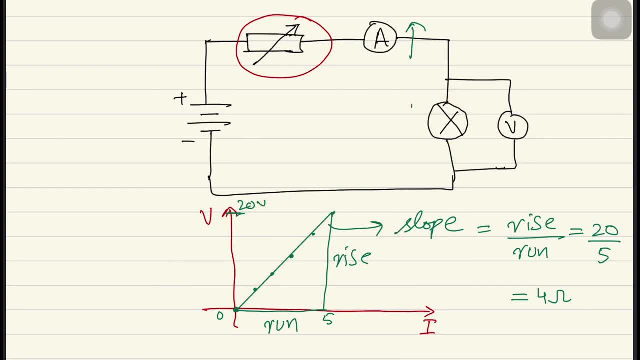 Okay, It will look like this. So we have current in the x-axis, We have the voltage in the y-axis, So the voltage will increase, but the current will not increase. So it will look like this, like that, Or if I switch the position of the voltage and the current, then our graph will look. 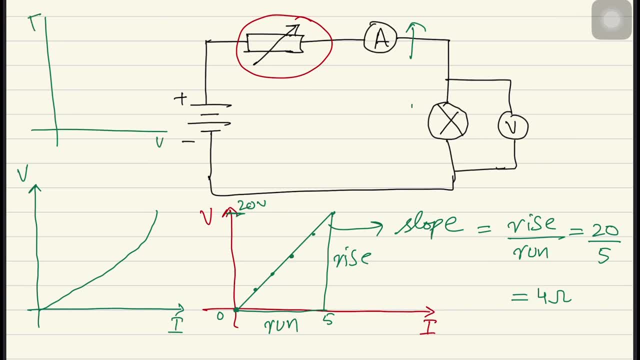 like this: If I keep voltage in the x-axis, current in the y-axis, Then our graph will look like this: There you go. So instead of going straight, you will see this curve in this graph. This shows that with the increase in current, the temperature increases. 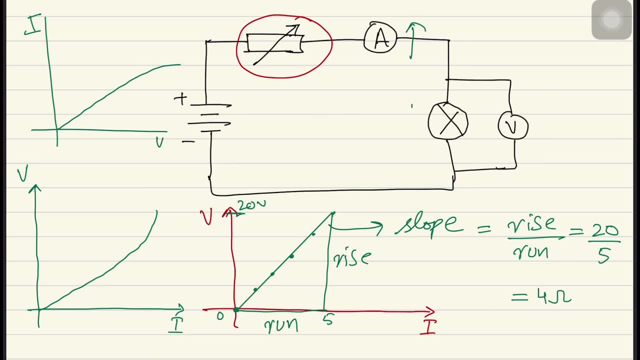 And when the temperature increases, resistance increases. And when the resistance increases, the current will not flow according, the current will not be directly proportional to the voltage. So instead of observing this straight line, We will observe this curve Which shows that this bulb is not. in this bulb, the voltage and current are not directly. 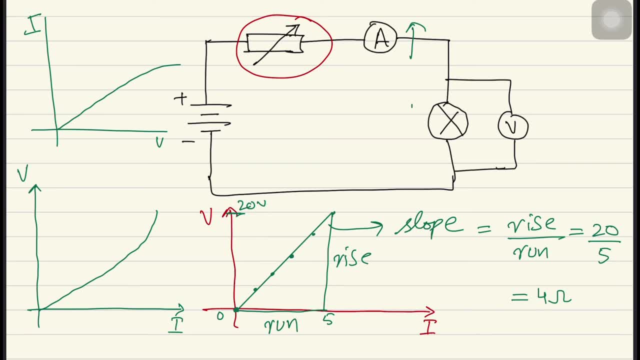 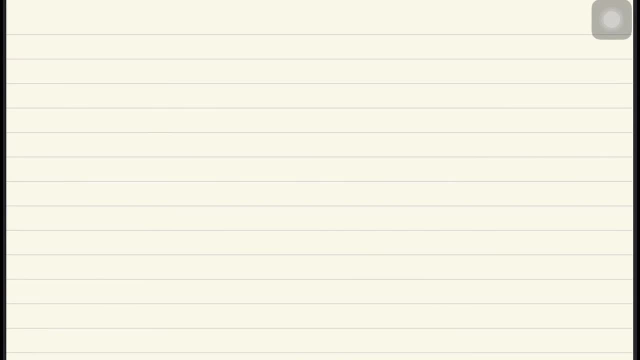 proportional to each other. Now, from here, I have to define a law that is called the Ohm's law. Okay, So let's define, let's come on to the Ohm's law. So, Ohm's law? Ohm's law is the basic, is the most basic law in the circuits. 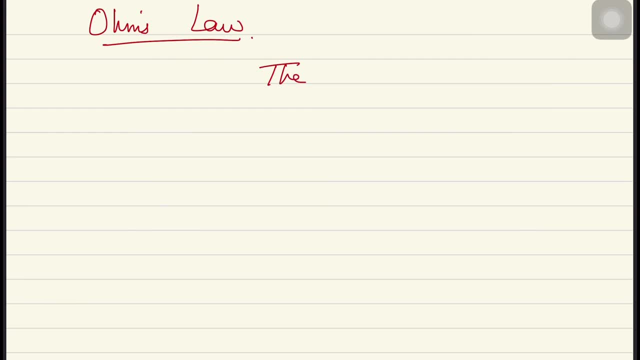 Ohm's law states that the current through a conductor is directly proportional to the voltage. Through a conductor is directly proportional to the voltage Through a conductor, is directly proportional to the voltage. Okay, So I can. and in the virtually proportional to the resistance. 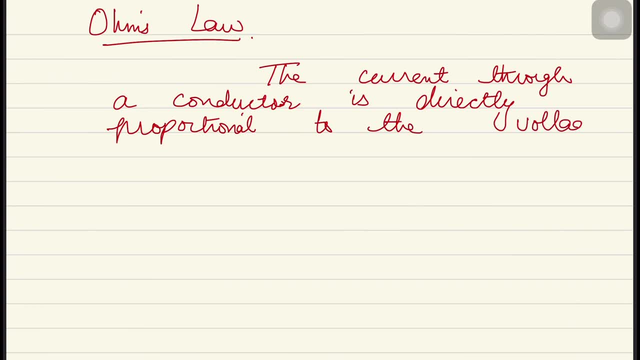 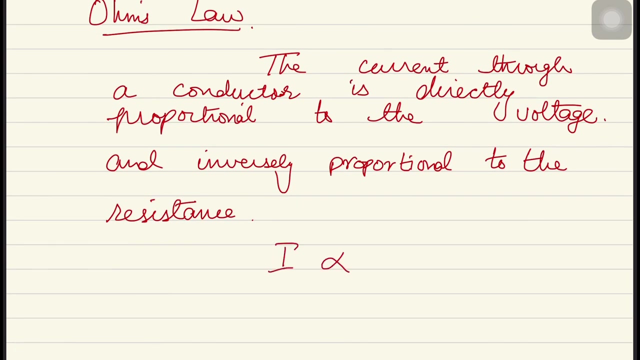 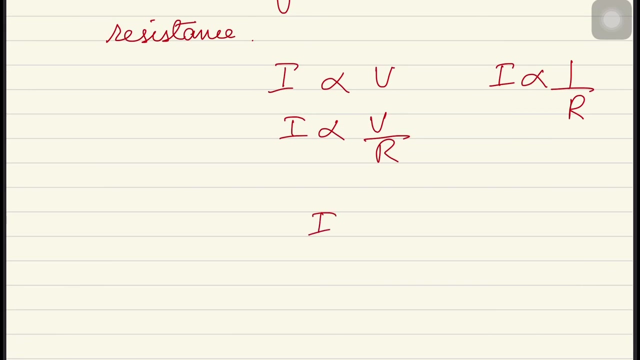 In the こちら Pres, which means that i can write it as like this: i is directly proportional to v, but i is inversely proportional to r, and when i'll combine it it will be look like i is proportional to v over r, or i can simply write it as i equals to v over r, or v is equal to. 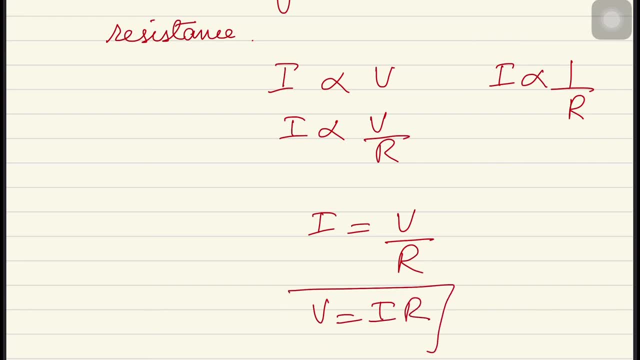 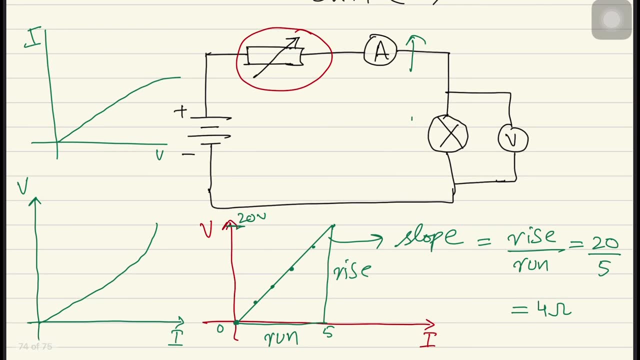 i r. so this is basically the ohms law now in this case of bulb, since the current and voltages are not directly proportional, so we'll say that this bulb is a non-ohmic conductor. why? because it is not following the ohms law. in place of this bulb, if you replace 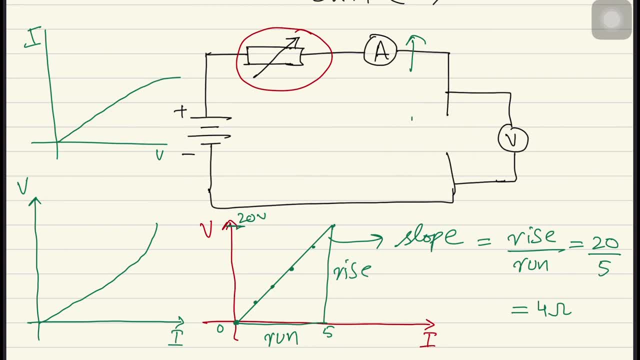 this bulb with a resistor. a resistor is basically an electrical component that has a fixed resistor and it is not affected by the temperature. okay, so that's a resistor. it is an electrical component that controls the flow of the current and its resistance is fixed and it is not affected by. 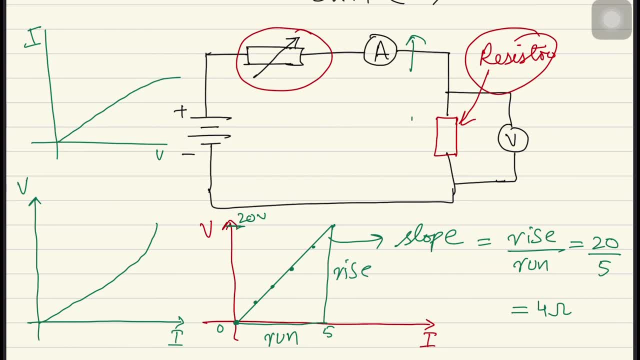 the temperature. so for this resistor we'll observe such a graph, a straight line: when we increase the current, the voltage increases. when we further increase the current, the voltage increases further. so we can say that this resistor is following the ohms law, because as you increase the voltage,